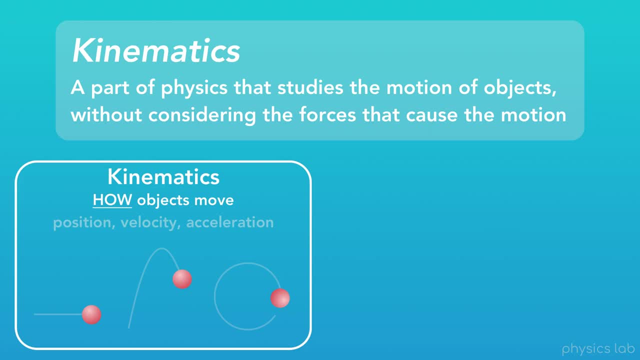 What direction is it going And how fast is it moving? On the other hand, dynamics focuses on why objects move or what causes them to move. This includes things like forces, energy, mass and momentum. When learning physics, we usually start with kinematics. 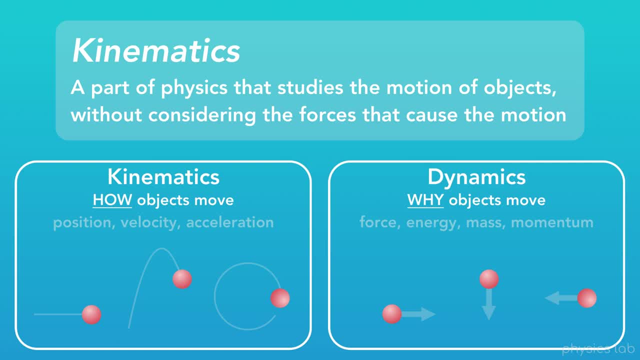 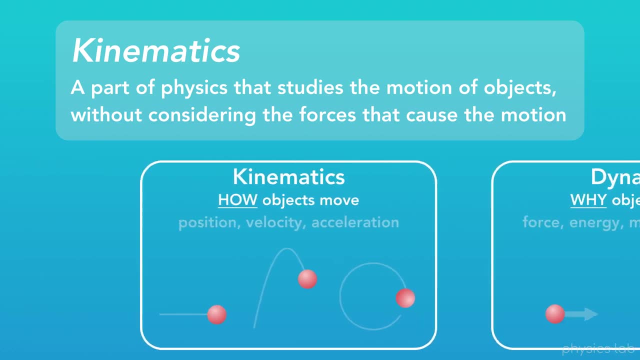 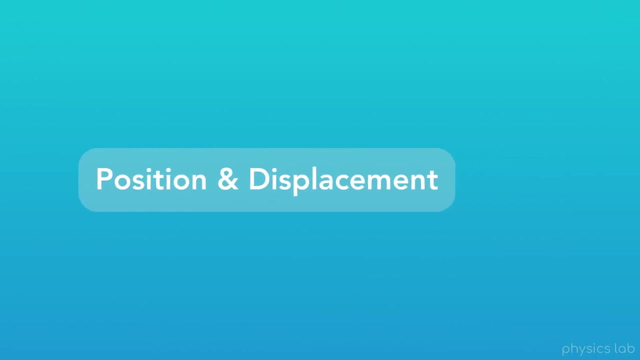 and learn how to describe the motion of objects first. Then in later sections we'll learn dynamics and what causes that motion. So let's get into kinematics First. we'll start with position and displacement. So position is pretty simple. We're going to describe position as where an object is. 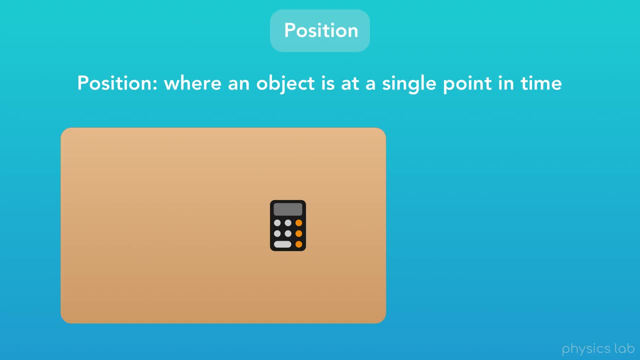 at a single point in time. For example, we might say the position of this calculator is on the desk, But the calculator could be any place on this desk. If we want to be more specific, we could say something like: The calculator is on the left side of the desk. 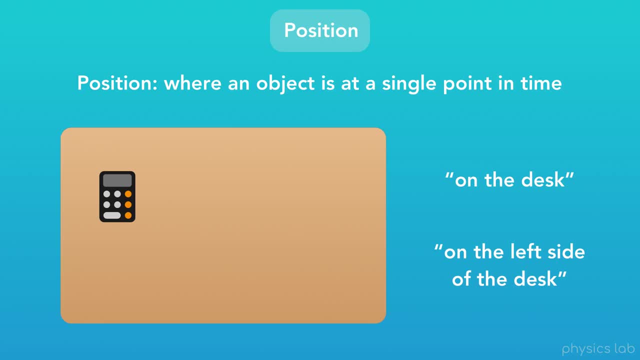 This is sort of how we're used to describing position in everyday life. As another example, here's a flag attached to a flagpole. How would we describe the position of the flag? Well, here we might say the flag is up, Or here we might say the flag is down. 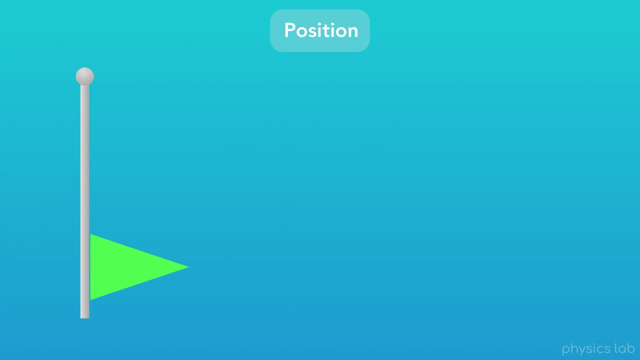 Again, this is how we would normally describe position, But in physics we need to be extremely specific about where things are. The laws of physics deal with exact positions and exact times. We can't plug things like up or down or the left side. 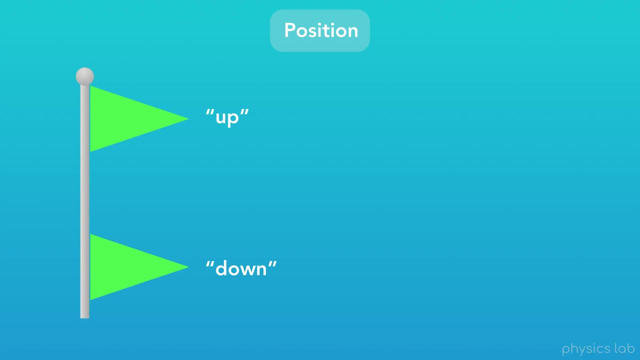 of the desk into our physics equations. So how do we be more specific? Well, we use numbers. If we were to hold up a tape measure, so the end is at the bottom of the flagpole- we can measure exactly where the flag is by using numbers. 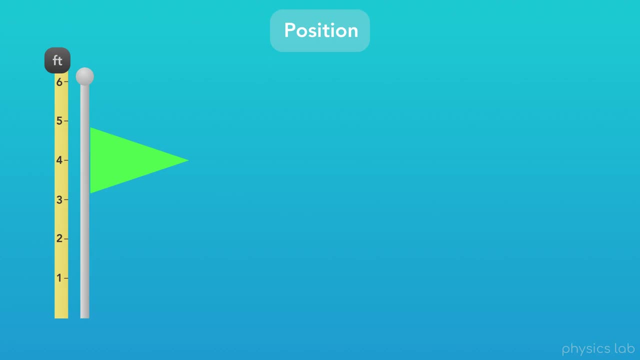 And since all objects have some length or width, we'll need to pick a point. So let's say we have a point on the object to measure. Most of the time we'll pick the middle. So let's measure from the middle of this flag. 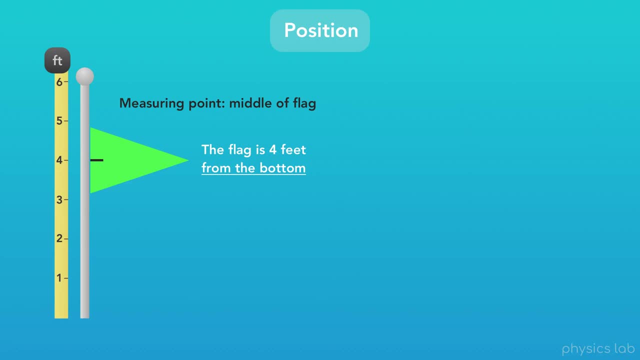 Now, instead of saying up or down, we can more precisely say: the flag is four feet from the bottom or the flag is two feet from the bottom. Now we're describing the exact position of the flag on this flagpole. Also, notice how we're measuring the position of the flag: relative. 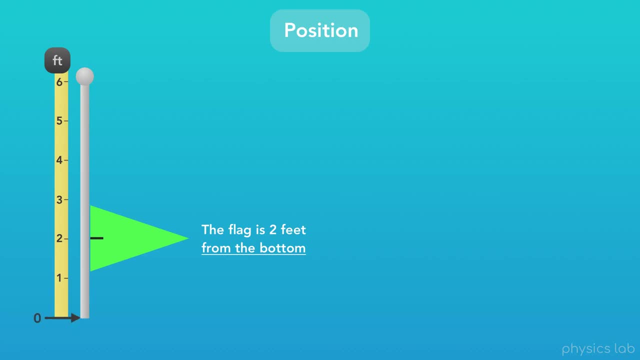 to the position of the flagpole, where the position would be zero. We always have to measure position relative to some point And we don't have to pick the bottom. What if we measured the position of the flag from the top? Now, the top of the flagpole has a position of zero. 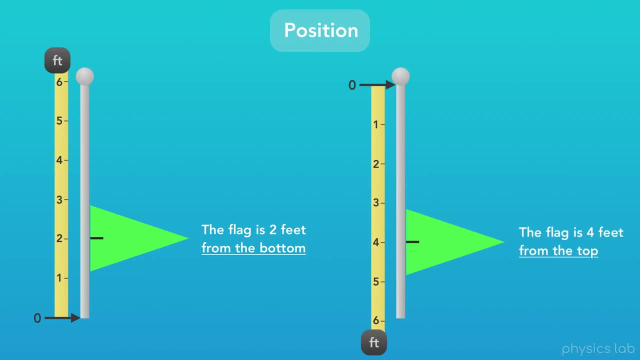 And if the flag was in the same position as it is on the left now, we would say: the flag is four feet from the top, And both ways of measuring are fine. All we need to do is pick our zero point that we're measuring from. 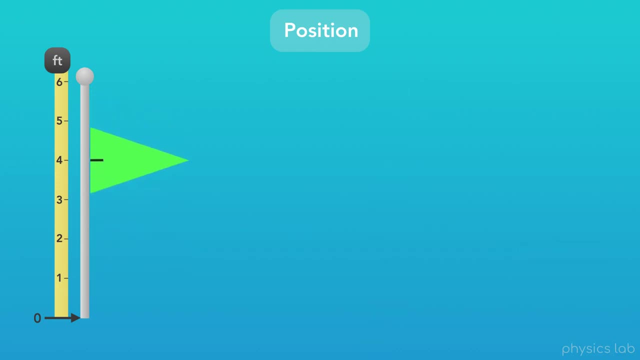 Now, since the flag can only move up or down this flagpole in a straight line. we're measuring position along one dimension. We can describe the position of this flag by using only a single number, like four feet, One-dimensional motion or linear motion. 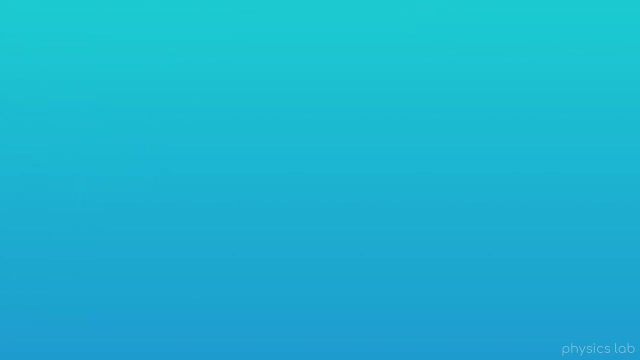 is what we'll be learning first. So as we start to talk about the position, velocity and acceleration of objects, I think it'll help if we stick with one real-world example that we can relate everything back to. So let's use a car driving along a flat, straight road. 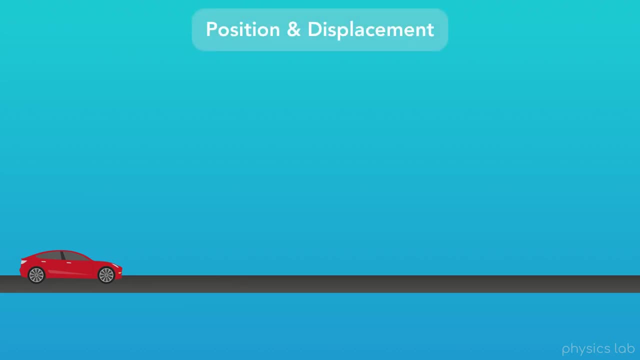 Just like we held a tape measure up to our flagpole to measure the position of the flag, we're going to use this number line to show the position of the car along the road. In physics, we represent the horizontal position of an object using the variable x. 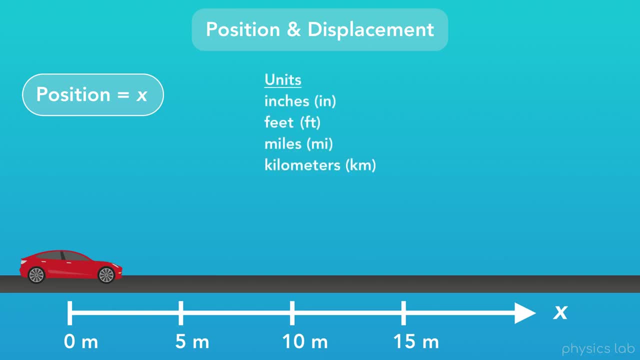 Position could have any unit of length or distance, such as inches, feet, miles or kilometers, But we'll be using the SI unit of position, which is meters, or lowercase m for short, As a reference. 1 meter is equal to about 3.3 feet. 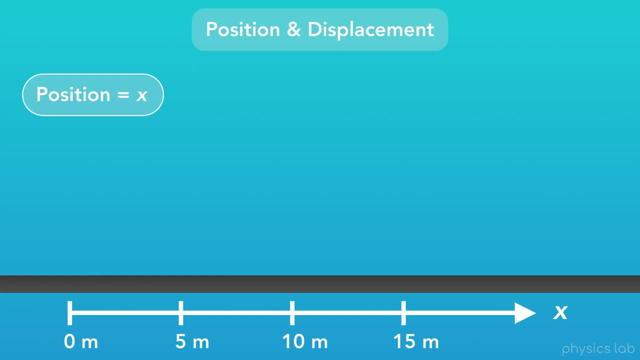 or about 1 yard. So let's say the car starts at a position of 5 meters, but then it drives to a position of 15 meters. This is what we call displacement. Displacement is the change in position of an object. 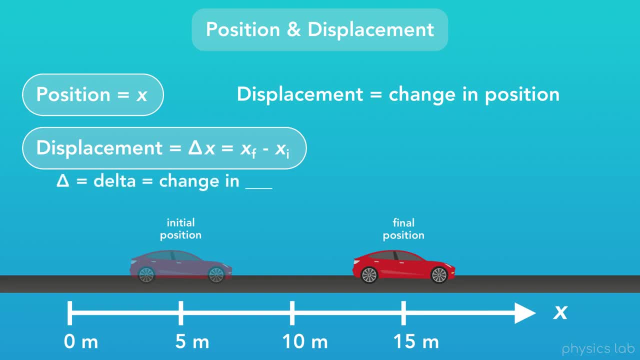 Here's our equation for displacement, And this little triangle here is called delta. It's a letter of the Greek alphabet and it means the change in something. So in this case it means the change in position, The way we actually calculate displacement. 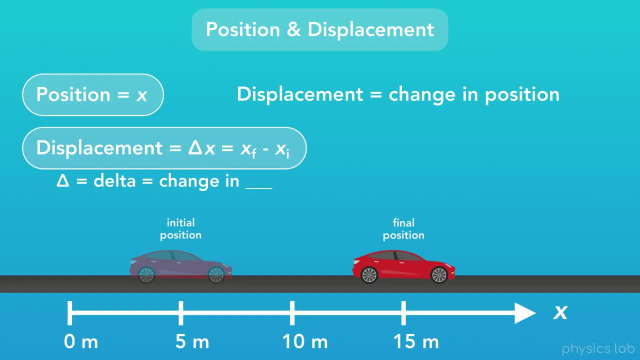 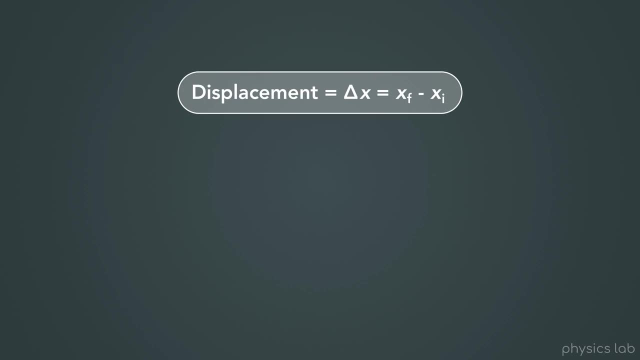 is the final position minus the initial position. Let's take a closer look at this So you'll notice, in this equation we have the variable x, which means position, but we also have these two variables, these tiny letters f and i. 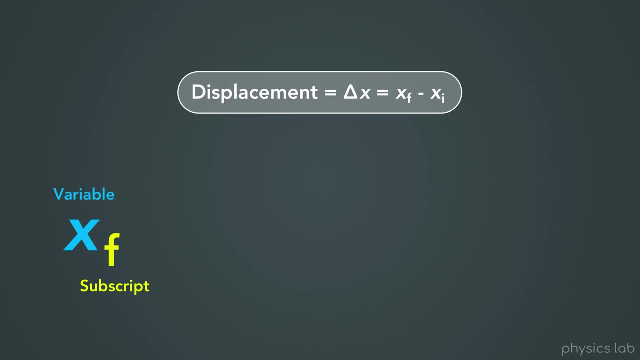 When we have a variable with a small letter or number at the bottom right, the larger letter is our variable and the small letter is called a subscript. The variable x means position and the subscript f means final. So together as a whole they mean final position. 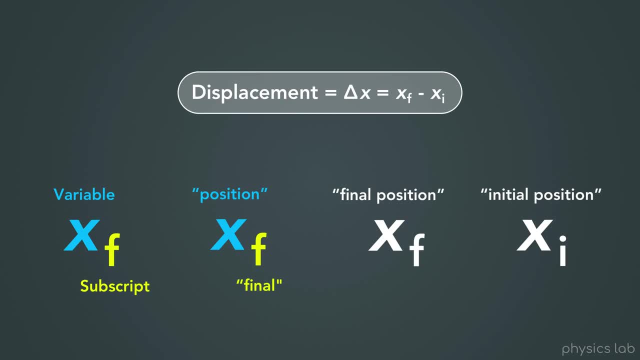 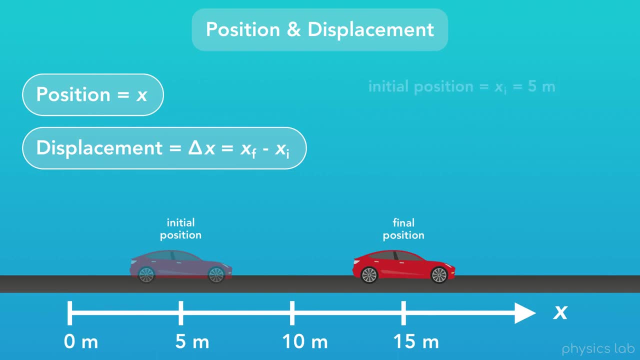 And x sub i or just xi, means initial position. So what was the displacement of the car? The initial position, or xi, is 5 meters and the final position, or xf, is 15 meters. From our equation we see that the displacement 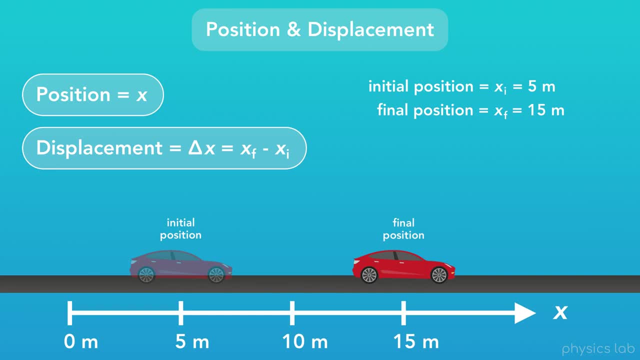 is the final position minus the initial position. So in our case that would be 15 meters minus 5 meters, which gives us 10 meters. So when the car drove forward, its displacement was 10 meters. So now that we have an idea of what position is. 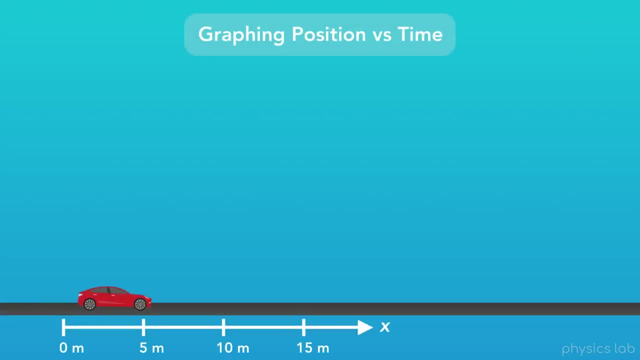 let's take a look at how we could graph the position of this car over time as it moves. To do that, we'll start by listing the position of the car at different points in time, as if someone was standing on the side of the road. 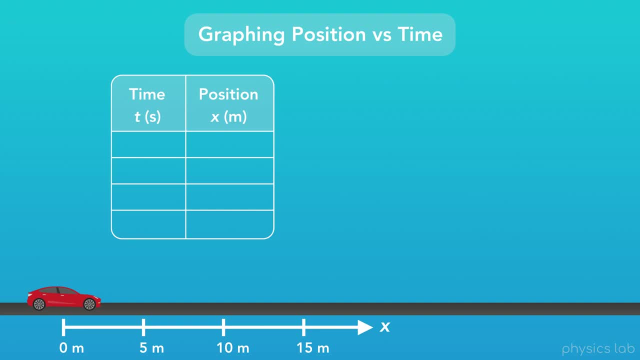 with a stopwatch and recording the position of the car at different times. So let's say the car is driving forward like this: At the very beginning the position of the car is 0 meters and after 1 second the car's position is 5 meters. 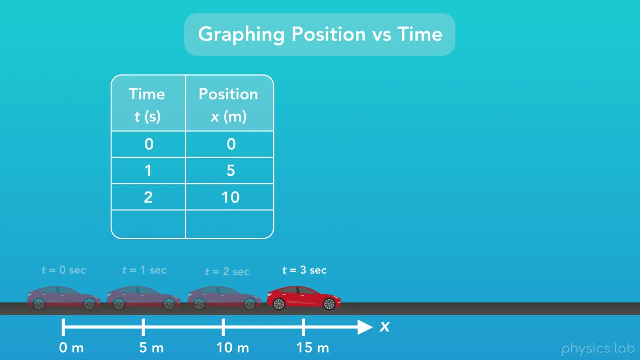 After 2 seconds, the car's position is 10 meters, and after 3 seconds the position is 15 meters. Now we have a table showing the car's position at different points in time. So what would a graph of the car's position over time look like? 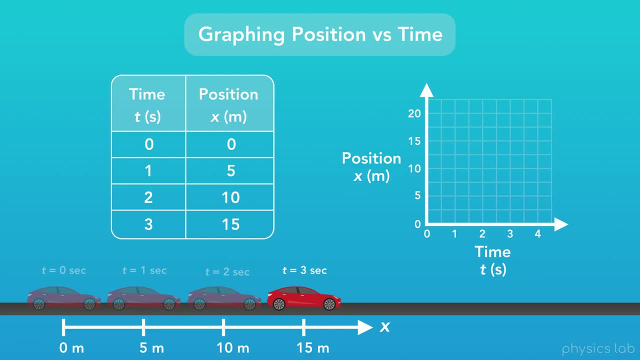 We'll start with an empty graph where the x-axis, or the horizontal axis, represents time and the y-axis, or the vertical axis, represents the position of the car on the road. Now it might seem weird that we're putting the car's 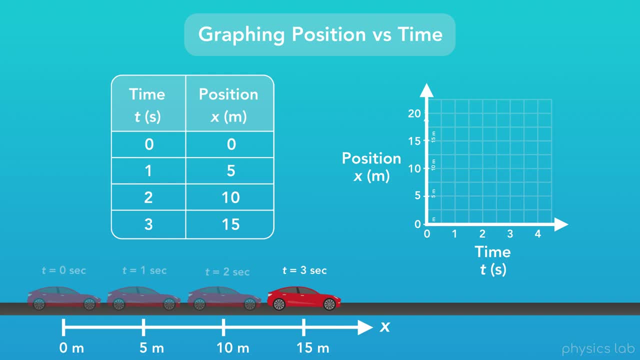 horizontal position on the vertical axis of the graph. but the reason is we always put time on the horizontal axis. That will make more sense throughout the course, but for now just know that we always put time on the horizontal axis of the graph. 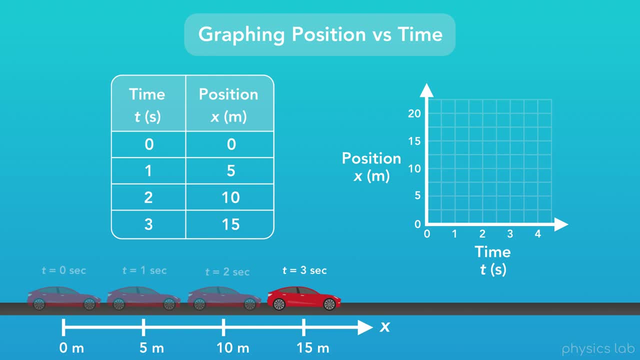 So how do we graph the position of this car over time? We start by plotting the points that we have in the table on the left. When time equals 0 seconds, the position of the car is 0 meters, so we'll plot that point on the graph. 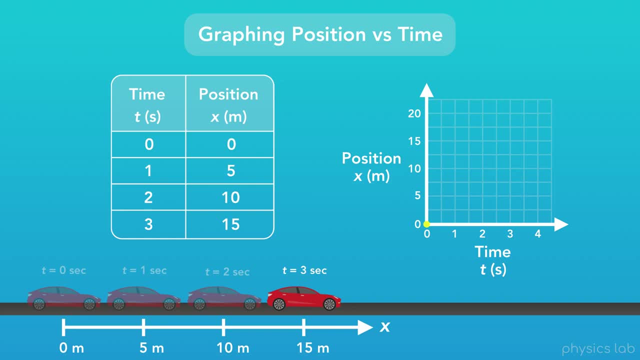 where time is 0 and position is 0.. Next, when time equals 1 second, the position of the car is 5 meters. so we'll plot the point where time equals 1 and position equals 5.. We also have points for when time equals 2 seconds. 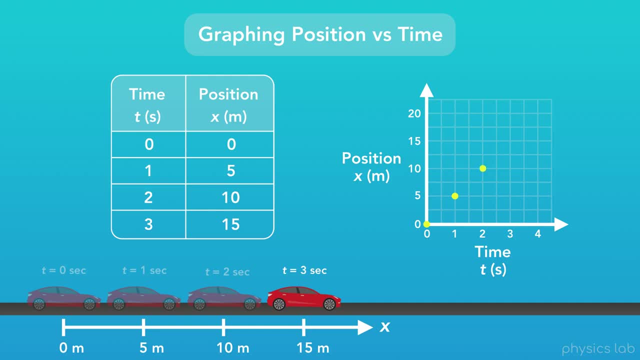 and the position is 10 meters, and when time equals 3 seconds and the position is 15 meters. Now that we have some data points on our graph, we can connect the points with lines like this, And there we go. 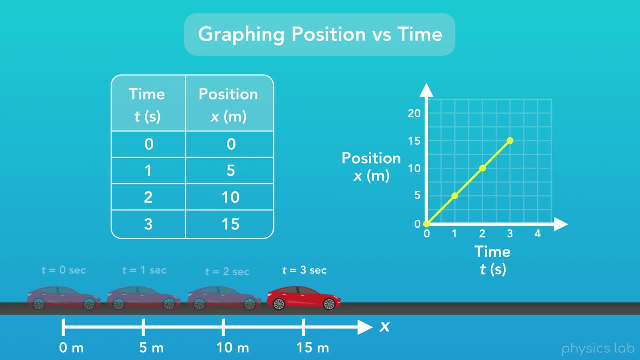 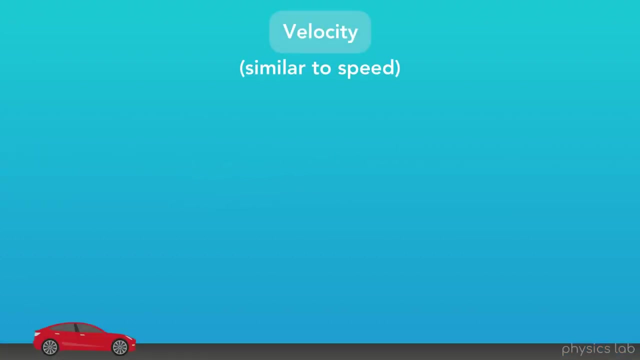 For this car's motion. we've graphed the position versus time, and now we have another way to visualize that motion. Next, let's talk about velocity. Velocity is similar to speed, but we'll talk about why it's different from speed later on. 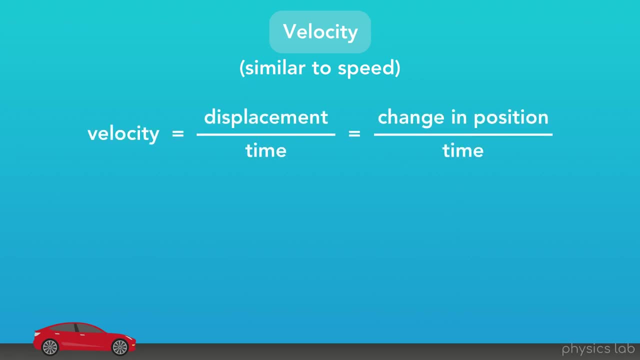 Velocity is defined as the displacement of an object divided by the amount of time it takes that object to travel, which is the same thing as the change in position over time. There are some common units we could use to describe velocity or speed, such as miles per hour. 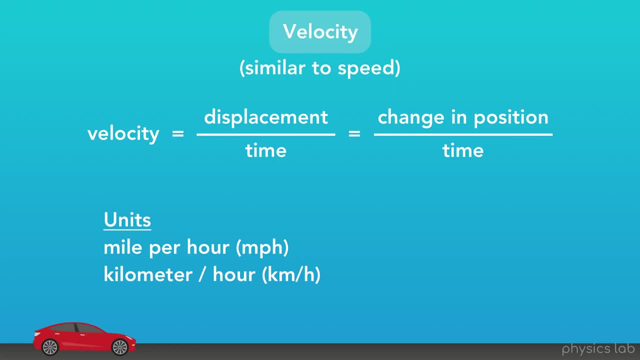 or kilometers per hour, But the unit we use in physics, the SI unit of velocity, is meters per second, abbreviated as m over s. For reference, 1 meter per second is roughly 2.2 miles per hour or 3.6 kilometers per hour. 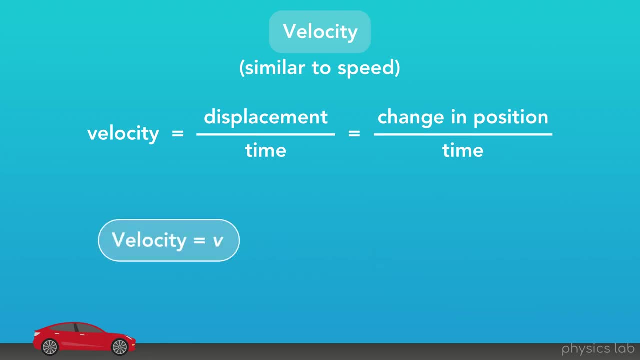 So we represent velocity using the variable v and we represent time using the variable t. So here's our equation for the average velocity of an object. We could say the average velocity equals the displacement over time, or we could write out each of the variables separately. 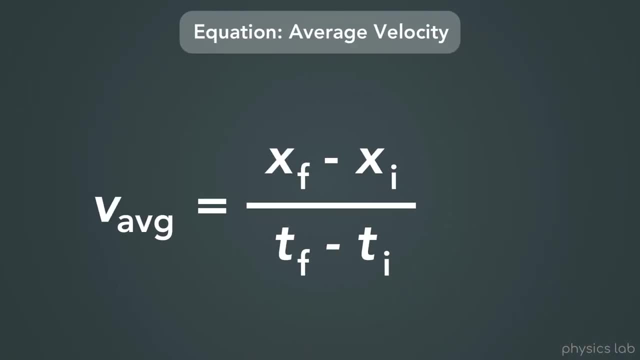 Let's take a closer look at this equation. So v with the subscript avg stands for average velocity, xf is the final position, xi is the initial position, tf is the final time and ti is the initial time. Altogether, this equation says: 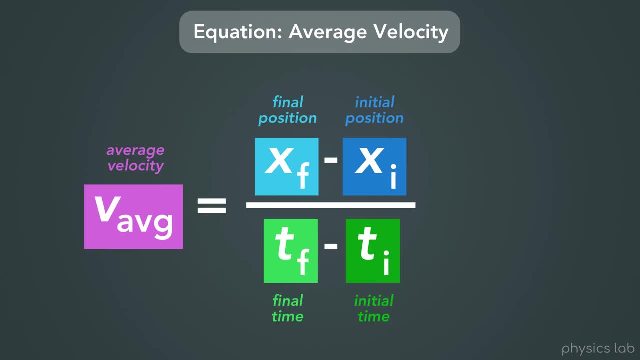 that the average velocity of an object equals the final position minus the initial position, divided by the final time minus the initial time. Another way to say it is: the average velocity equals the change in position over the change in time. And here are the SI units. 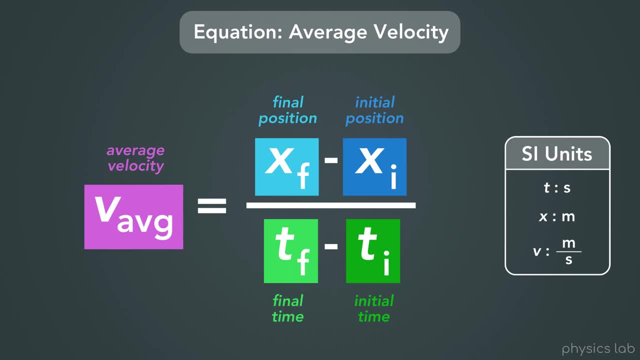 for the variables in this equation: Time is in seconds, position is in meters and velocity is in meters per second- An important thing when we use physics equations like this one. the math only works out if we plug in numbers using SI units. 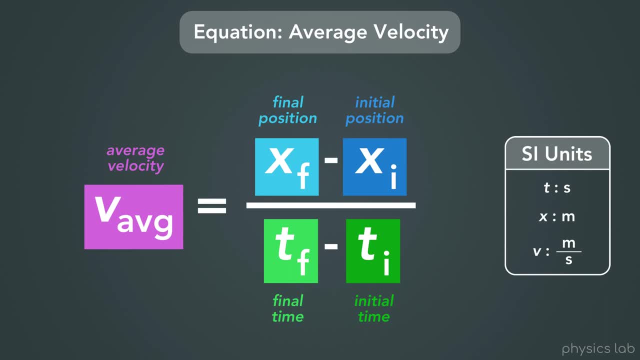 We can only get velocity in meters per second if we plug in position in meters and time in seconds. Of course you could use any units you want, like inches and hours, but then your velocity will be in inches per hour and things could get a little crazy. 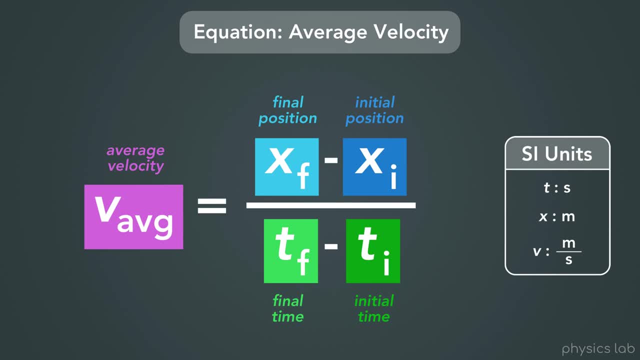 especially if you're using multiple equations in a problem. So just remember to stick with the SI units when we're using equations. And one more thing I want to note here is that this equation that we just learned is the same thing as this equation. 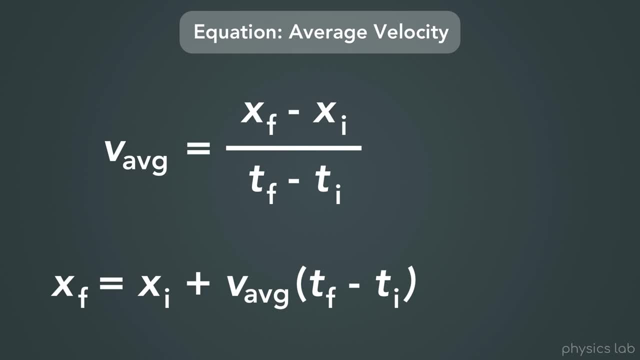 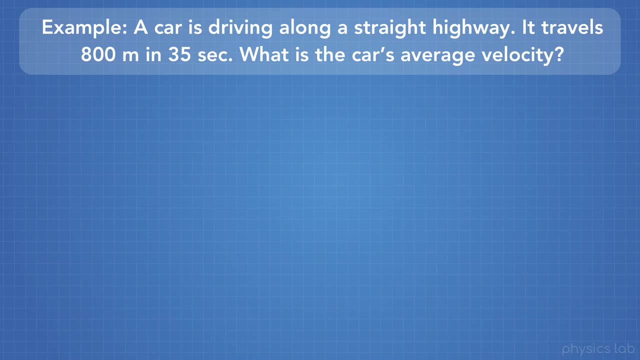 You might see this equation in class or on an equation sheet. These are the exact same equation, but the variables have just been rearranged Alright, so let's do an example problem to try out this equation. A car is driving along a straight highway. 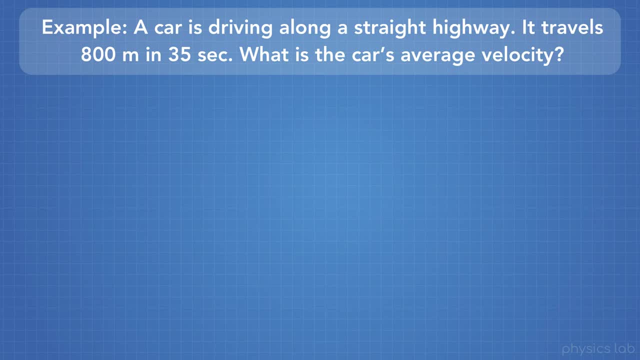 It travels 800 meters in 35 seconds. What is the car's average velocity? First, let's draw a picture to see what this looks like. It's pretty simple: We just have a car on a straight road and it travels 800 meters. 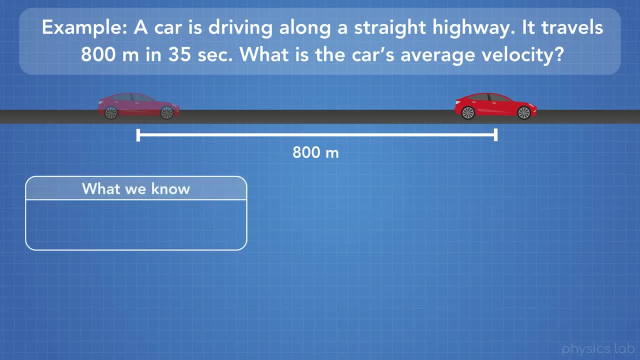 Next we're going to write down what we know For this problem. we know that the change in the car's position or the displacement of the car is 800 meters. We also know that the change in time is 35 seconds. 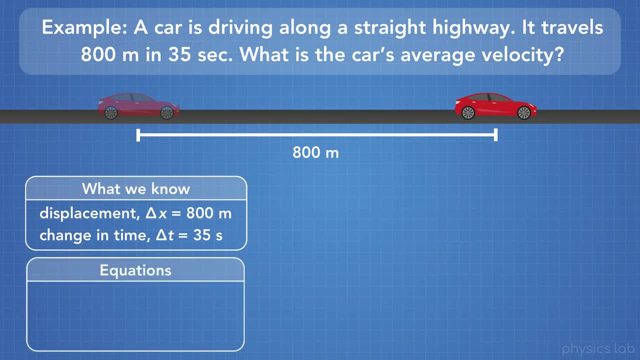 Next, we'll list out the equations that we might be able to use. Since this problem wants us to find average velocity, we'll use the equation that we just learned. Since we know the displacement and the change in time, we can just use the first part of our equation. 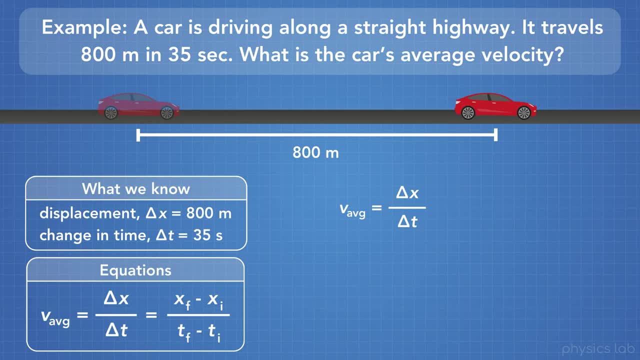 Average velocity equals displacement divided by change in time. We would plug in 800 meters for the displacement and 35 seconds for the change in time. And don't forget that we always need to keep track of our units. Using our calculator, we'll do 800 divided by 35,. 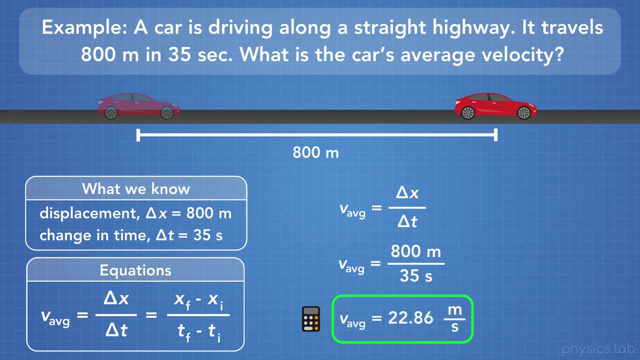 and we'll find that the average velocity equals 22.86 meters per second. And just a side note: sometimes we might write our units using a fraction like this, and sometimes we'll write it out all in one line by using a slash. 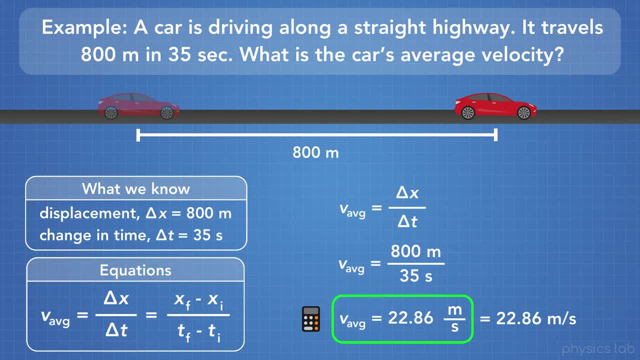 So you might have asked: why didn't we use the other part of our equation with the initial and final variables? Well, we can try that too. Here we're using the equation: average velocity equals the final position minus the initial position, divided by the final time minus the initial time. 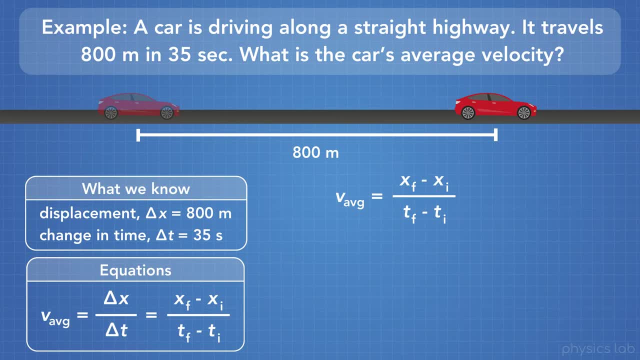 The question is: where do we plug in our 800 meters and 35 seconds? Well, since the problem doesn't say what the initial position of the car is or what the initial time is, then we're always going to assume that the initial values are zero. 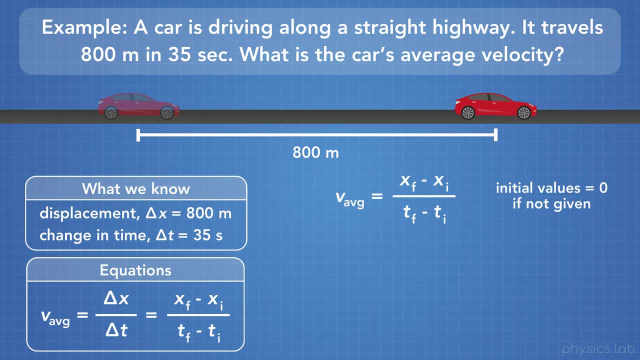 if they're not given In this case, our picture might look a little bit different. Now we can see that the car has values for its initial position and for its final position. At the initial position, we assume that time equals 0 seconds. 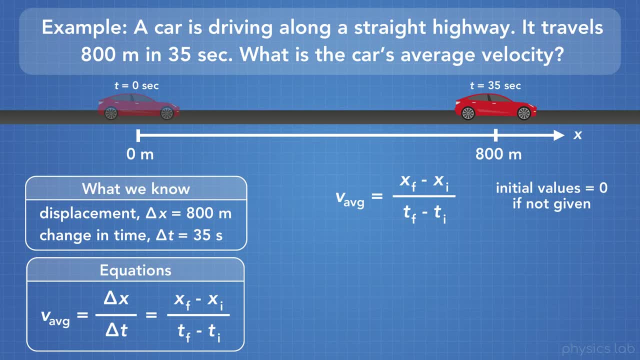 and the position is 0 meters At the final position. time is 35 seconds and the position is 800 meters. Now we can plug in: 800 meters for the final position, 0 meters for the initial position, 35 seconds for the final time. 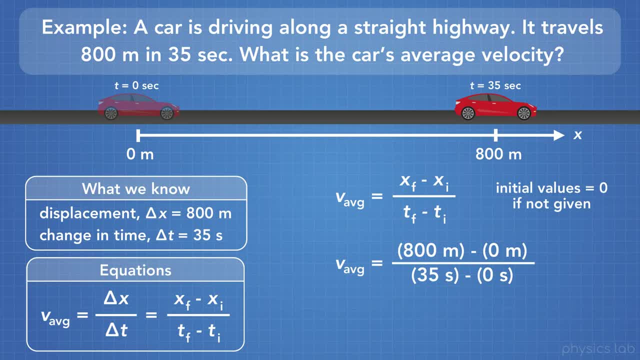 and 0 seconds for the initial time. And don't forget your units: 800 minus 0 is 800, and 35 minus 0 is 35. Now what we're left with is the same equation as last time, and we find that the average velocity of the car 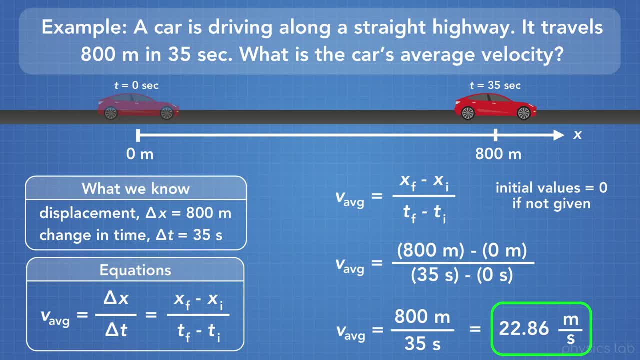 is 22.86 meters per second, So we could have done this either way. The thing to remember is that if we're not given an initial value, we have to assume the initial value is 0. But what if we are given both the initial and the final values? 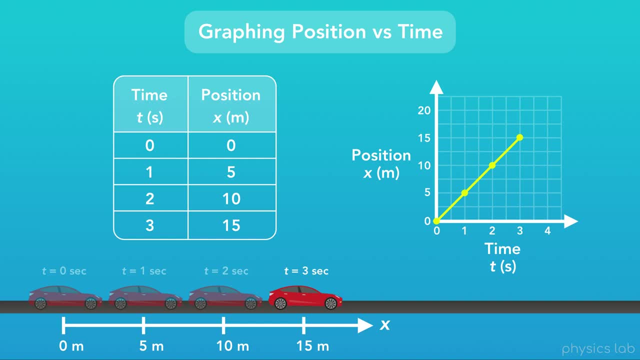 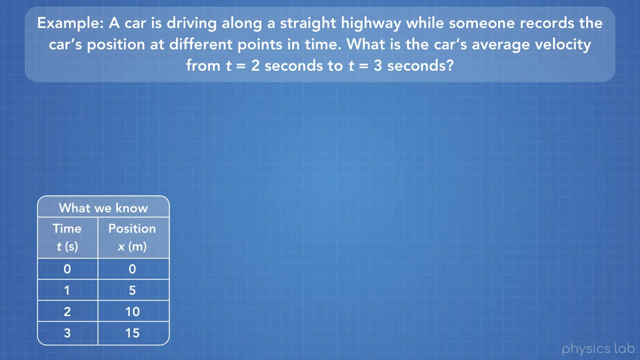 Let's use the example from when we made a table of a car's position at different points in time. So here's the new problem: A car is driving along a straight highway while someone records the car's position at different points in time. That's where we get our table from. 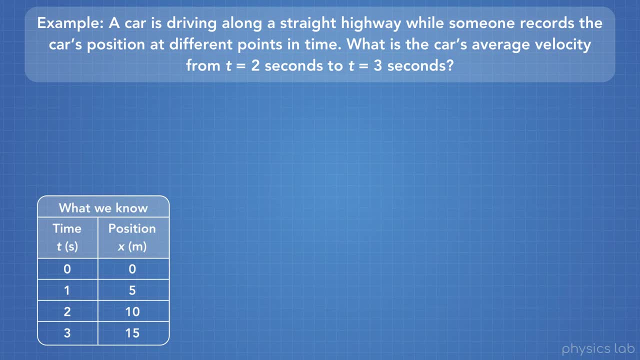 What is the car's average velocity from when time equals 2 seconds to time equals 3 seconds? First, here's a picture of this scenario. Next, we're going to write down what we know. In this case, we're given the table. 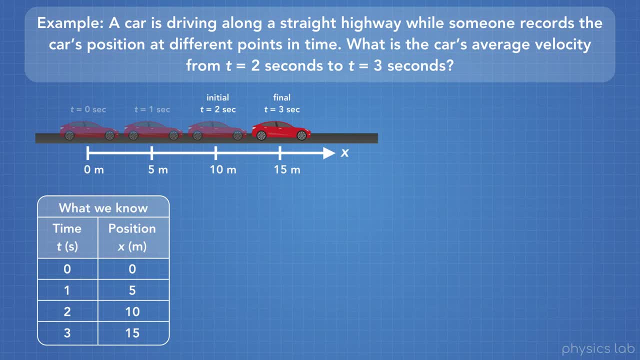 of the car's position at different times. Next, we're going to write down the equations that we could use to solve the problem, But this time we're specifically given an initial point and a final point, so we'll have to use the second part of our equation. 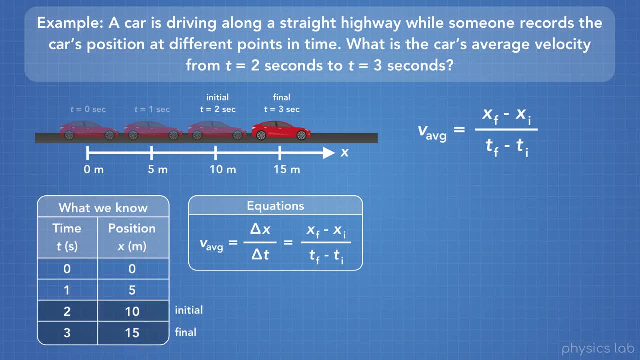 Our initial point is when time equals 2 seconds and the car's position is 10 meters. And the final point is when time is 3 seconds and the position is 15 meters. Now in our equation we can plug in 15 meters. 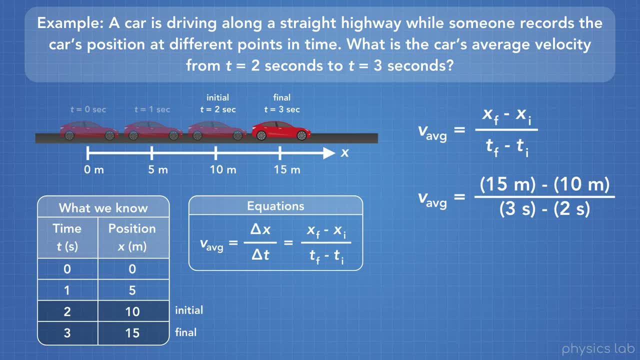 for the final position, 10 meters for the initial position, 3 seconds for the final time and 2 seconds for the initial time. 15 minus 10 gives us 5 meters and 3 minus 2 gives us 1 second. 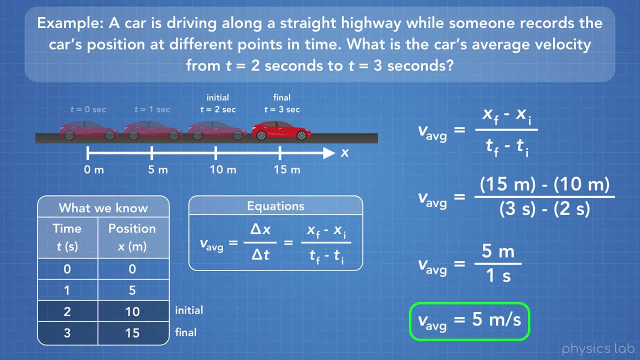 5 divided by 1 gives us 5,, so the average velocity of the car between these two points is 5 meters per second. So those are ways we could use the equation for average velocity. So, just like we did with position. 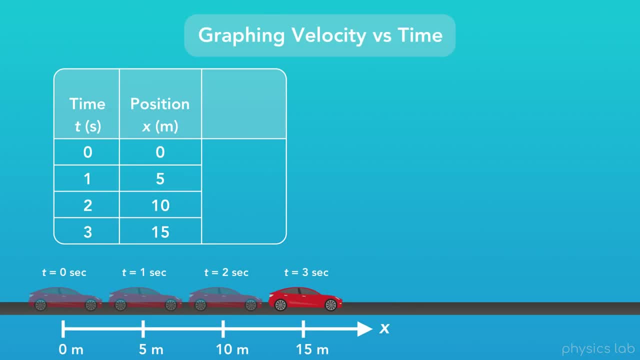 let's see if we can graph a car's average velocity over time. We'll use the same motion of the car moving from when we graphed the position, and then we can use the same data points that we had for the times and positions of the car. 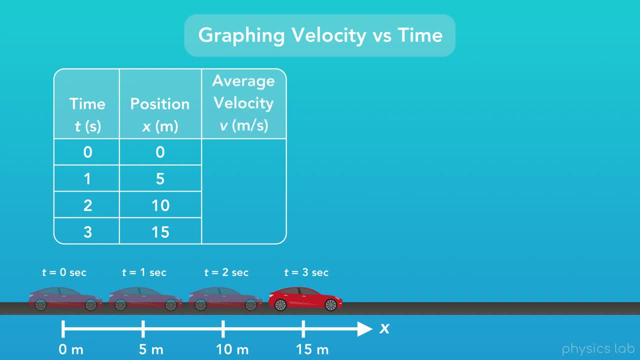 What we're going to do is calculate the average velocity of the car as it travels between each of these positions using our equation for average velocity. Between the first and second positions, the average velocity equals 5 meters minus 0 meters divided by 1 second minus 0 seconds. 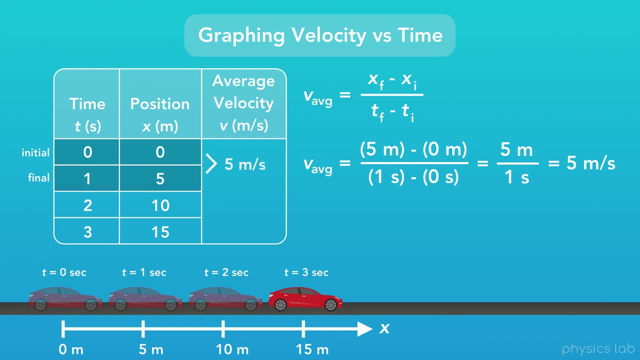 which gives us 5 meters per second. Between the second and third positions, the average velocity equals 10 meters minus 5 meters divided by 2 seconds minus 1 second, and that gives us 5 meters per second again. And last, between the third and fourth positions. 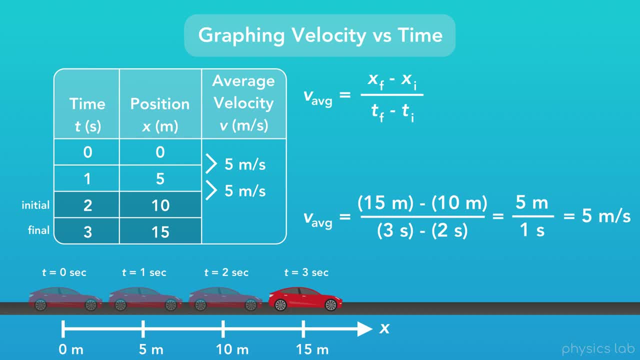 the average velocity is 15 meters minus 10 meters, divided by 3 seconds minus 2 seconds, which again gives us 5 meters per second. Alright, great. so now let's graph that Again, the horizontal axis will represent time. 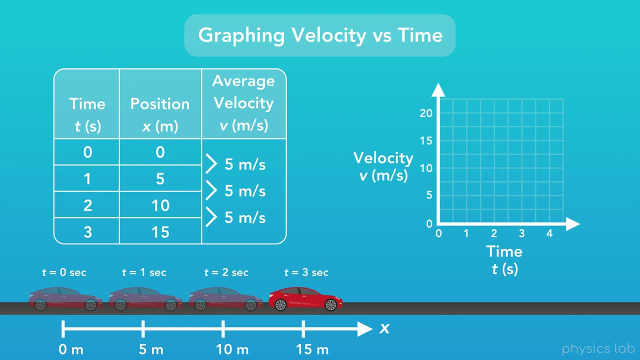 but this time the vertical axis is going to represent the velocity of the car. Now notice how each of these average velocities that we found do not correspond to a specific time point. We didn't calculate that the car was traveling 5 meters per second. 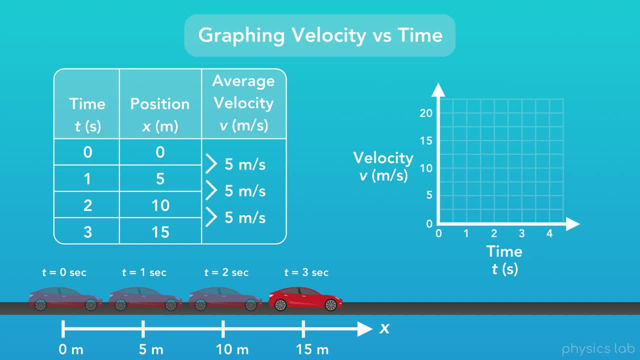 at exactly 1 second or 2 seconds. We only found the average velocity of the car as it traveled between two points. So instead of plotting points on our graph, let's just draw lines for each of these time intervals. This isn't how you would normally graph things. 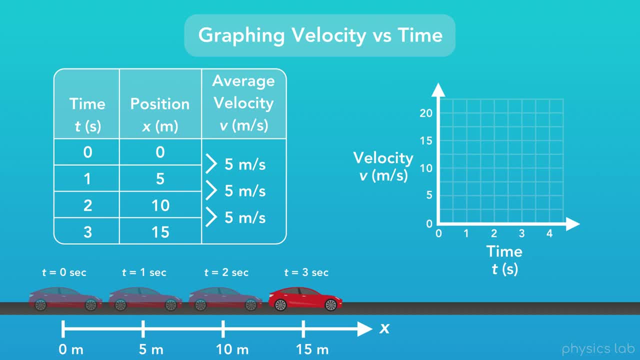 but we'll clear that up in a second. So, as the car traveled from 0 seconds to 1 second, the average velocity was 5 meters per second, and the same thing is true from 1 to 2 seconds and 2 to 3 seconds. 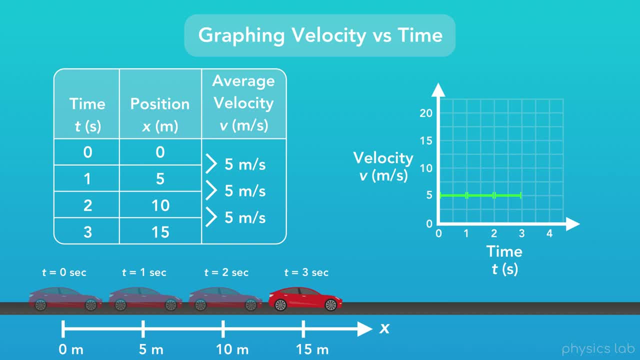 So here's a nice graph that lets us visualize the average velocities that we found. But what did we graph exactly? We were given the car's position at different points in time. Then we found the car's average velocity as it drove between each of these points. 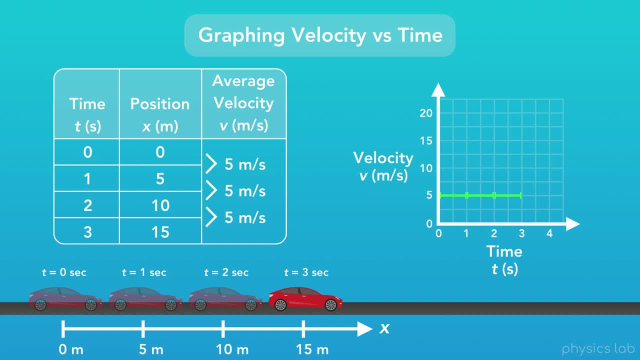 Then we plotted that average velocity across each time interval And it appears that the car is traveling at a constant 5 meters per second the entire time. But do we know that for sure? When you're driving, your speed might vary a little bit, right? 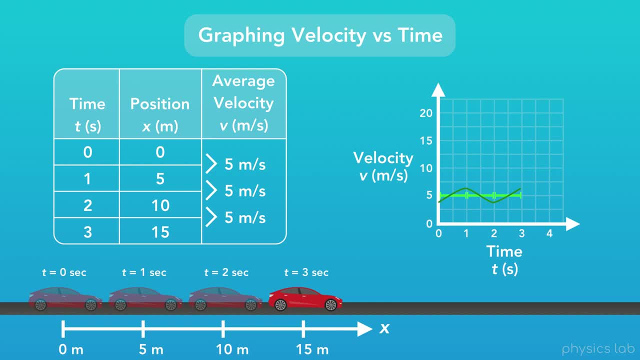 Is it possible that the car's velocity went up and down like this, but the average for each time interval was 5 meters per second? That actually is possible, but we don't know because we didn't graph the car's true velocity at every single instant in time. 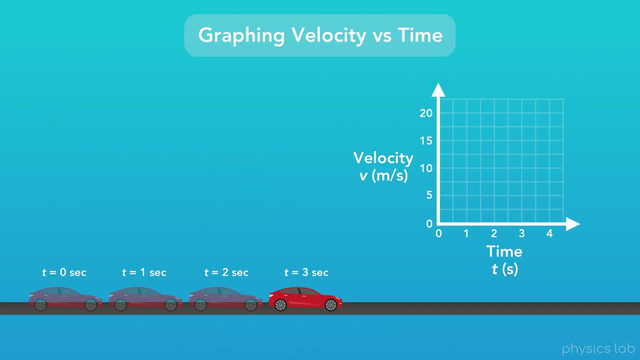 only the averages. So how could we do that instead? Well, every car has a speedometer which tells the driver how fast the car is moving. Usually it's in units of miles per hour or kilometers per hour, But for this example, 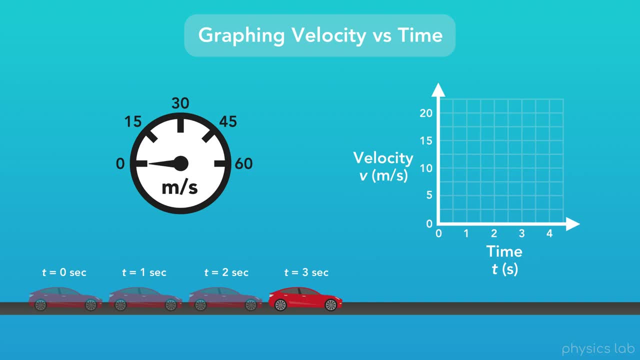 let's say the speedometer reads in meters per second. What if one of the passengers in the car watched the speedometer and wrote down the car's velocity at different points in time? At the start of this journey they noticed the speedometer reads 5 meters per second. 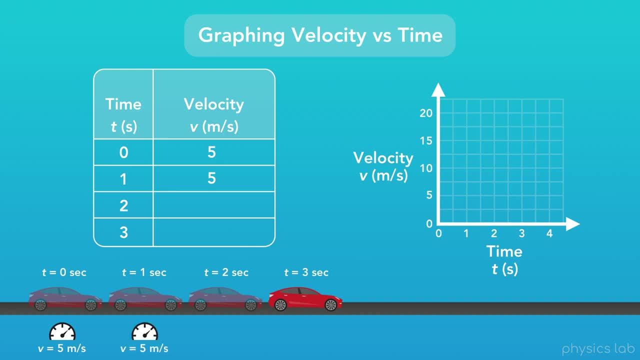 At exactly 1 second, they noticed that it reads 5 meters per second again. And at 2 seconds it reads 5 meters per second. And at 3 seconds it still reads 5 meters per second. Now what we have is a table. 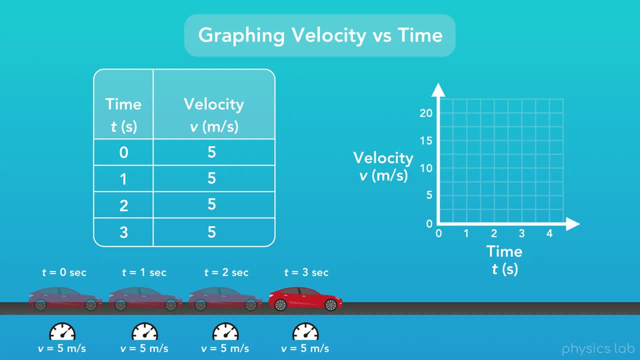 showing the car's true velocity at specific points in time, and this is what we call the instantaneous velocity. That means the car's velocity at any specific instant. This is different than when we found the car's average velocity between time points. However, since the car's velocity 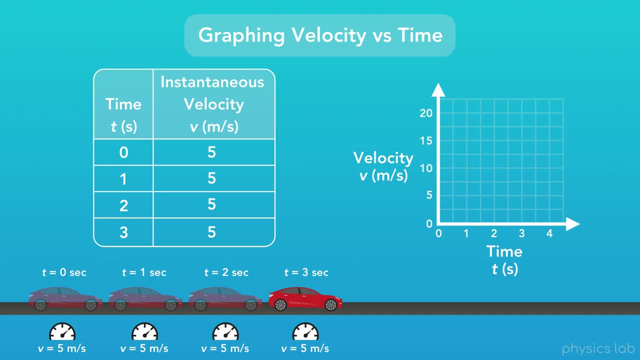 actually didn't change over time. it turns out that the instantaneous velocities are the same as the average velocities, So now we can graph the instantaneous velocity and each point in our table corresponds with one point on the graph. At 0 seconds, the velocity is 5 meters per second. 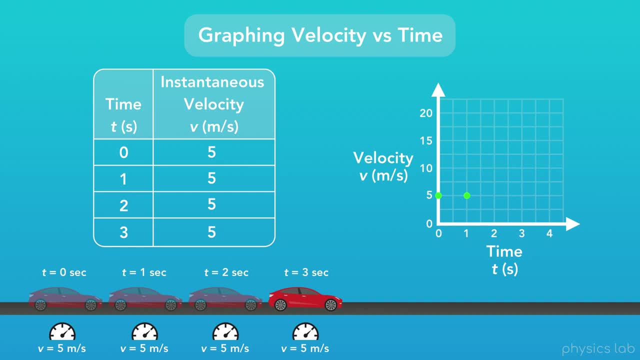 At 1 second it's still 5 meters per second, And at 2 seconds and 3 seconds the velocity is still 5 meters per second. Now we can connect our data points with a line and we have a graph of the car's. 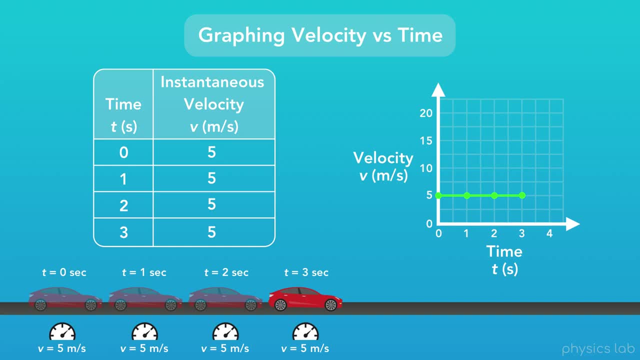 instantaneous velocity over time, And if the person in the car had recorded velocity every half second, we could add more points to our graph, and so on until we have a graph of the car's true instantaneous velocity at every single point in time. 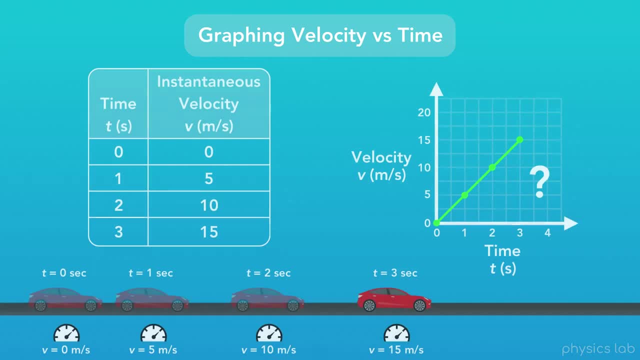 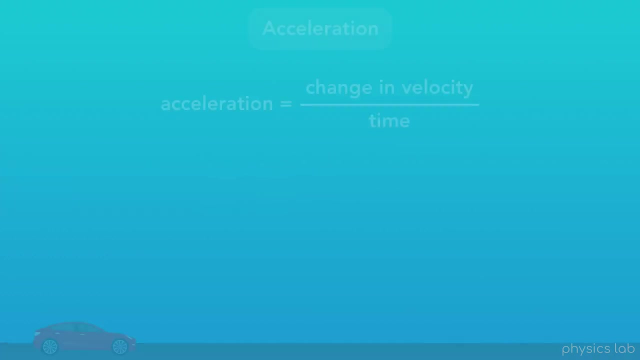 So here's a question: What would the car have to do so that the velocity graph increases over time Like this? Well, for that we would need acceleration. Acceleration is defined as the change in velocity of an object over time. 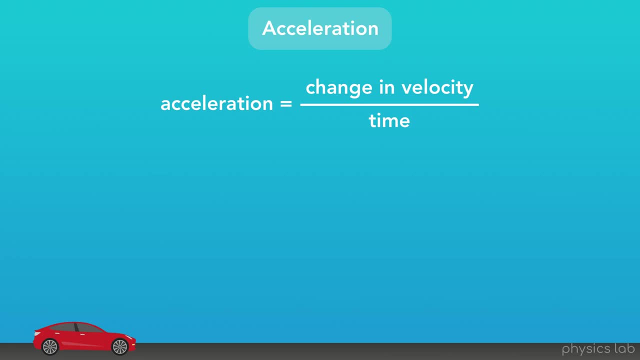 Acceleration might seem a little bit less relatable than velocity, but it's still something that most of us are used to. If you've ever heard someone say something like my car can go 0 to 60 in 4 seconds, well, they're talking about acceleration. 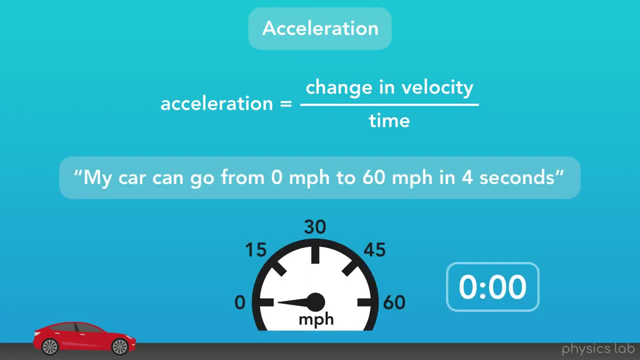 and acceleration. What they're really saying is: my car can go from 0 miles per hour to 60 miles per hour in 4 seconds. That means the acceleration of the car is its change in velocity, which is 60 miles per hour. 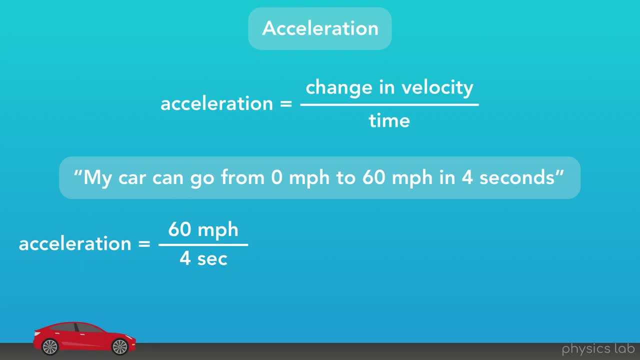 over the period of time, which is 4 seconds. 60 divided by 4 is 15, so the acceleration of their car is 15 miles per hour per second. That's the same as saying my car can go 15 miles per hour faster every second. 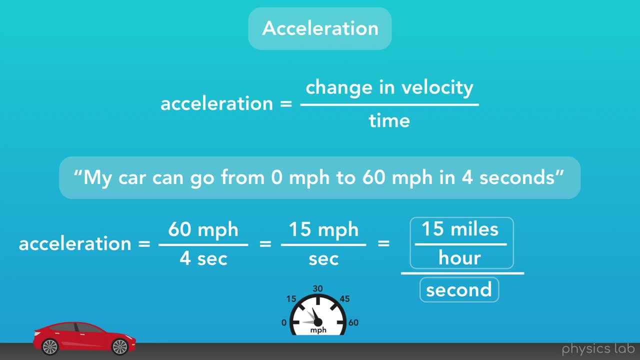 When the car is accelerating. after every second that passes, the speedometer moves up another 15 miles per hour, And this unit might look strange, but that's what acceleration is: Velocity miles per hour divided by time, seconds Written another way: 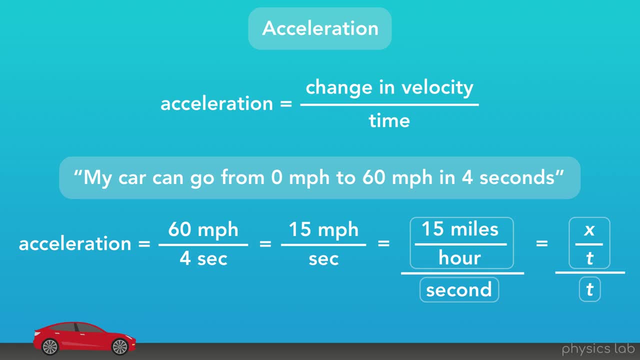 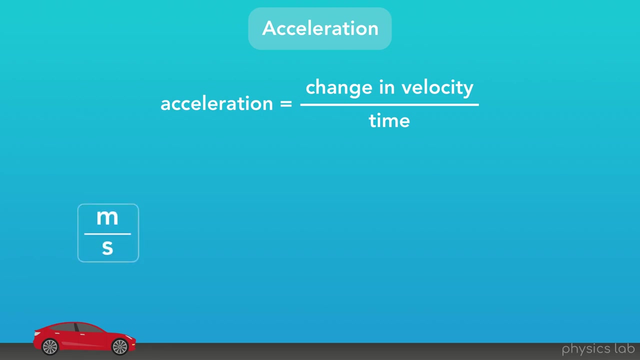 the unit of acceleration is a unit of position per unit of time, and that whole thing per unit of time. So what would the SI unit of acceleration be? Well, our SI unit of velocity is meters per second and our SI unit of time is seconds. 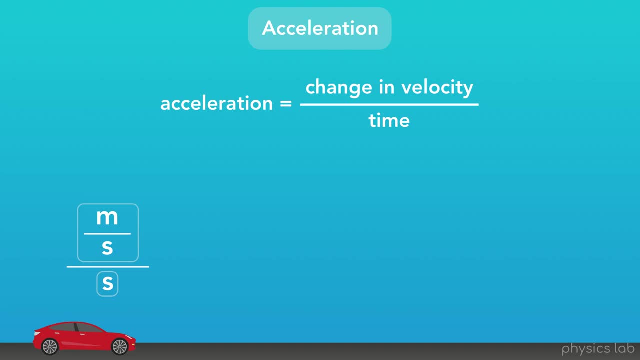 So this unit would be meters per second. per second, Mathematically, that's actually the same as meters divided by seconds times seconds, which is the same as meters divided by seconds squared. And that's our SI unit for acceleration: meters per second squared. 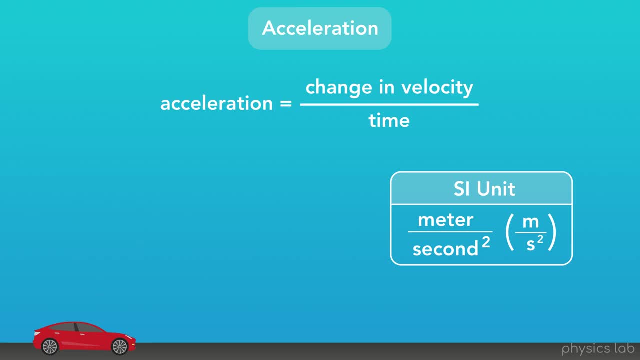 abbreviated m over s squared, And we'll be representing acceleration with the variable a. So a car is one example of an object that can accelerate. What's another example? Well, it turns out that if you drop an object like a ball, 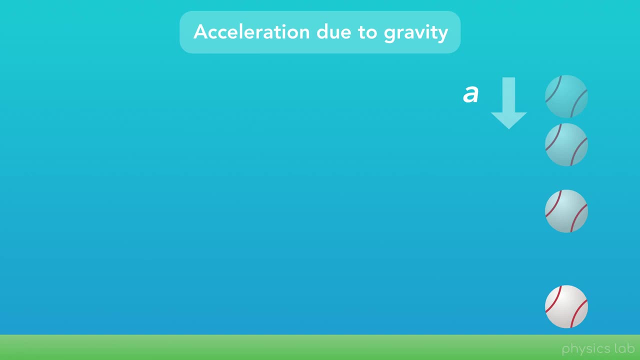 it'll actually accelerate as it's falling. This is what we call the acceleration due to gravity. We don't need to understand gravity yet or why this happens, but it's a good time to mention that all objects that are falling with gravity have the exact same acceleration. 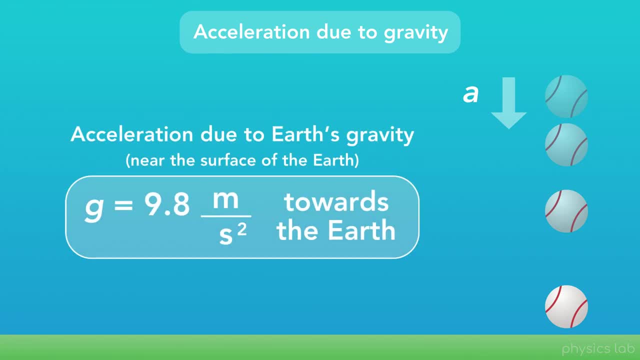 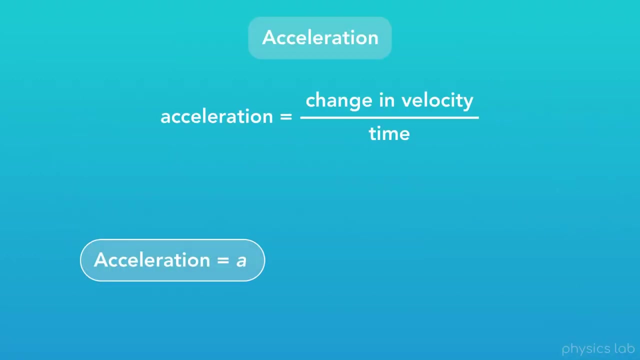 This acceleration due to Earth's gravity is 9.8 meters per second squared towards the Earth, And we represent this special value using the variable lowercase g. We'll leave it at that for now and we'll come back to it later. So how do we calculate acceleration? 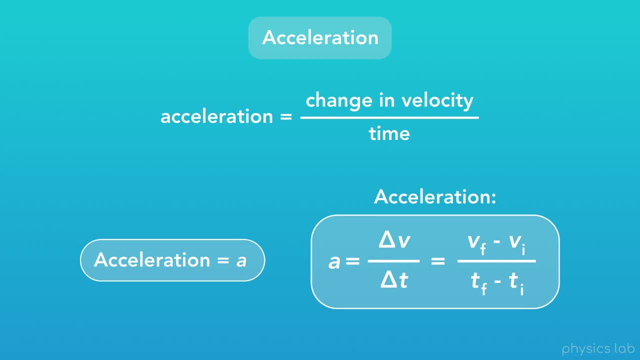 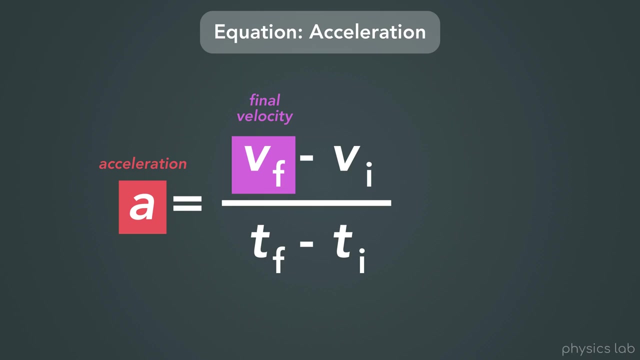 Here's our equation: Acceleration equals the change in velocity over the change in time. You might notice it looks similar to our equation for average velocity. Let's take a closer look. So a stands for acceleration. vf is the final velocity, vi is the initial velocity. 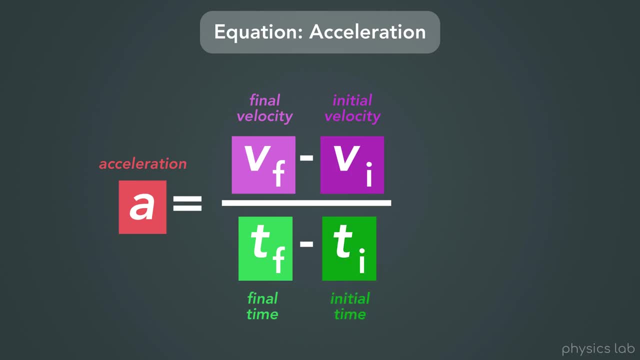 tf is the final time and ti is the initial time. So this equation says that the acceleration of an object is the final velocity minus the initial velocity, divided by the final time minus the initial time. Another way to say it is: the acceleration is the change in velocity. 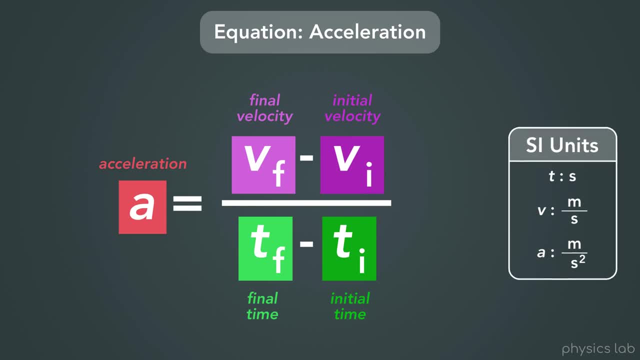 divided by the change in time. And here are the SI units for the variables in this equation: Time is in seconds, velocity is in meters per second and acceleration is in meters per second squared. Also, although it's not super important, I do want to mention that, just like our equation, 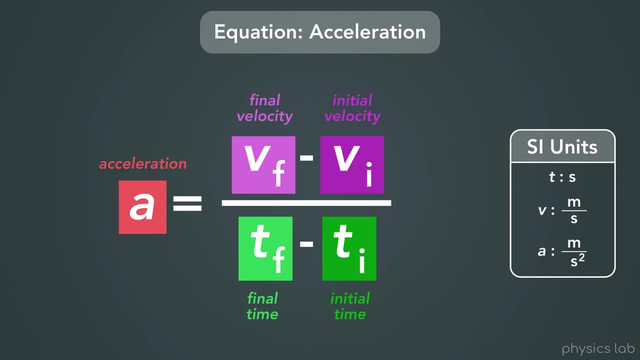 for average velocity. this here is really the equation for average acceleration, But we won't be dealing with changing accelerations in this course, so the acceleration at any time will always be the same as the average acceleration. Also, it seems that most classes and equation sheets 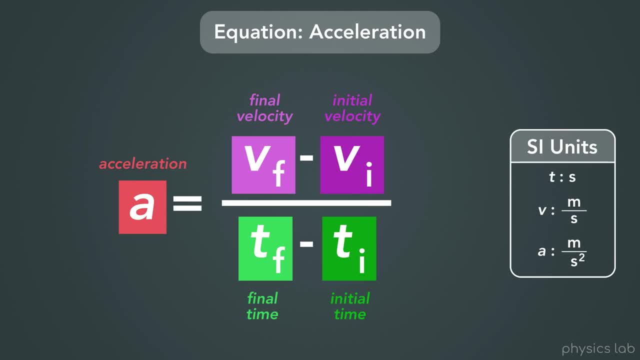 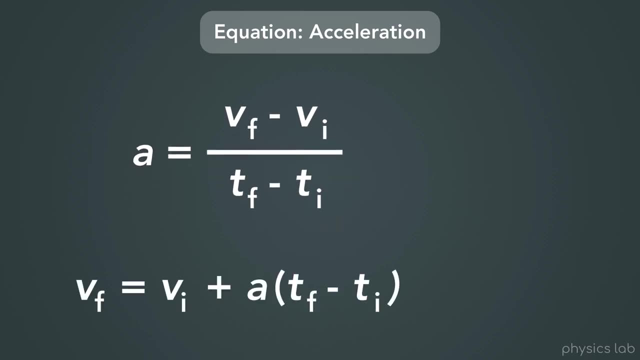 just call this acceleration. so that's what we're going to do in this course And, like before, you might see this equation written a different way, like this: These two are the exact same equation, but with the variables rearranged in different ways. 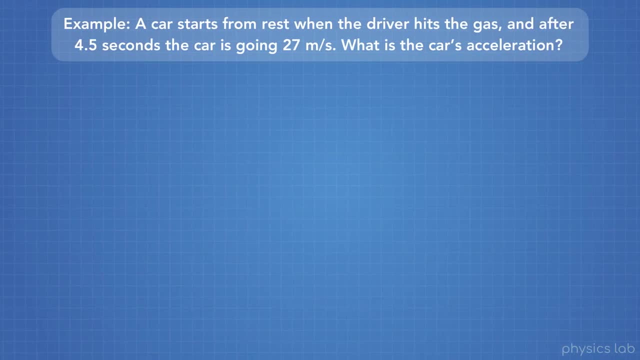 So let's try an example problem. A car starts from rest when the driver hits the gas and after 4.5 seconds the car is going 27 meters per second. What is the car's acceleration? So first we'll draw a quick picture. 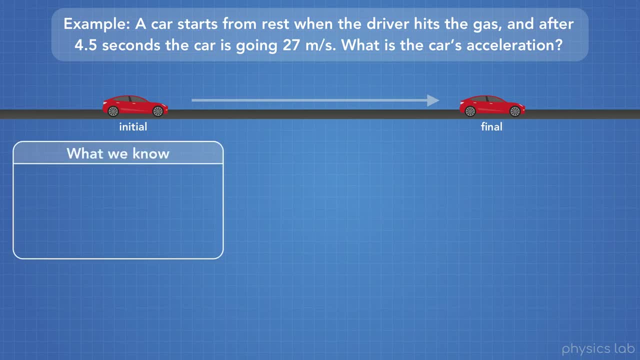 just to see what it looks like. Next we need to write down what we know. The problem says that the car starts from rest. In physics, when we say an object is at rest, that means that it's not moving and therefore its velocity is zero. 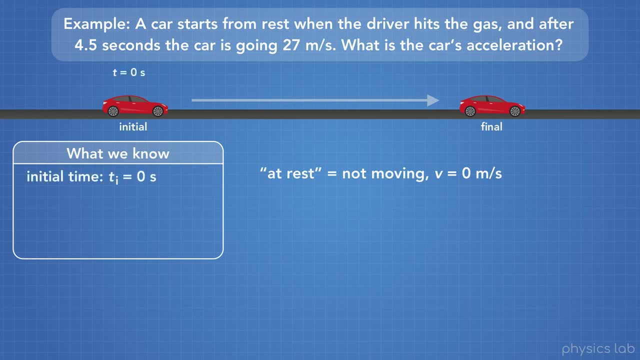 So we'll say that at the initial point, when no time has passed, that the initial time is zero seconds and since the car started from rest, the initial velocity is zero meters per second. We also know that at the final point. 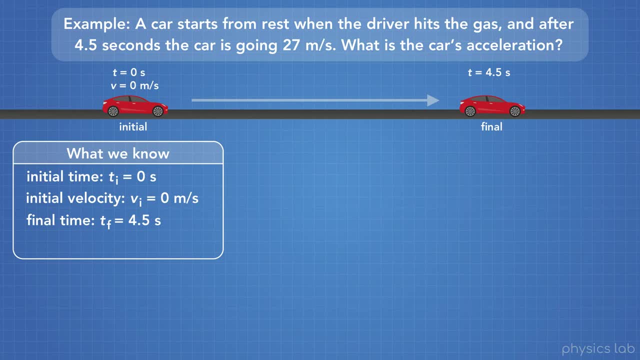 the final time is 4.5 seconds and the final velocity is 27 meters per second. After that, we write the equations that we might use for this problem, and here we're looking at our equation for acceleration, Since we have an initial and a final velocity. 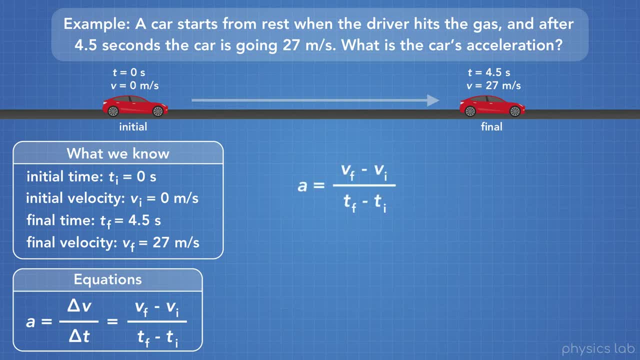 let's use the right part of this equation. So acceleration equals the final velocity minus the initial velocity, divided by the final time minus the initial time. Next we'll plug in the variables that we know. The final velocity is 27 meters per second. 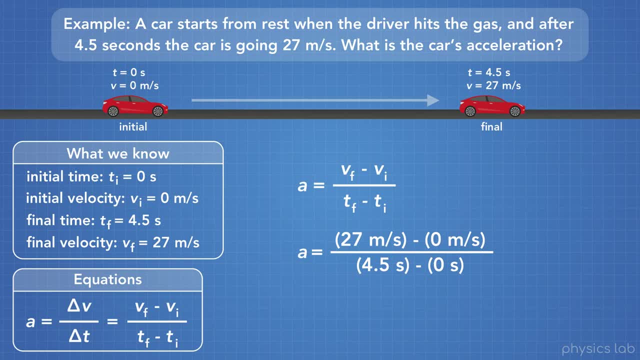 and the initial velocity is zero meters per second, The final time is 4.5 seconds and the initial time is zero seconds. And don't forget to keep track of your units. I usually find it easiest to write it out like this: 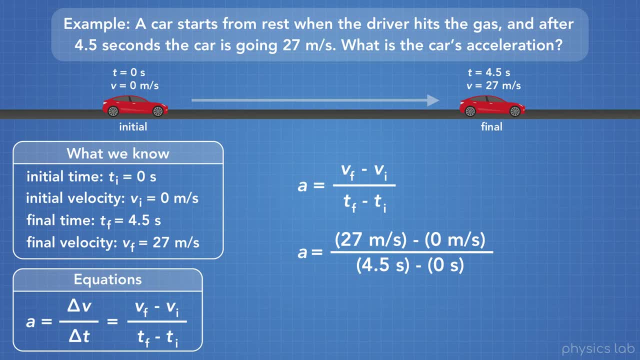 with each number and its unit in parentheses, so that I can keep them together. If this looks a little confusing, here's just the math that we're doing: 27 minus zero, divided by 4.5 minus zero. If we plug that into our calculator, 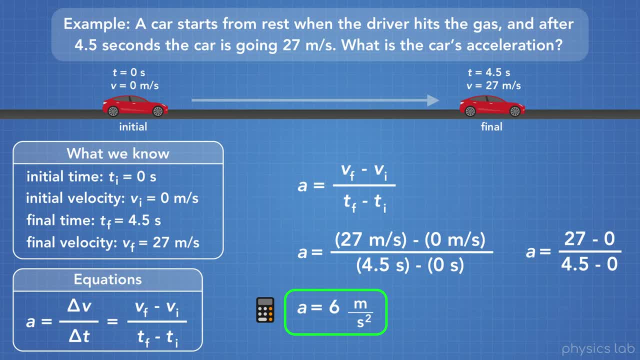 we find that the acceleration of the car is 6 meters per second squared. We know the units for our answer, because we know the SI unit for acceleration is meters per second squared and we have followed the rule of only plugging the correct SI units. 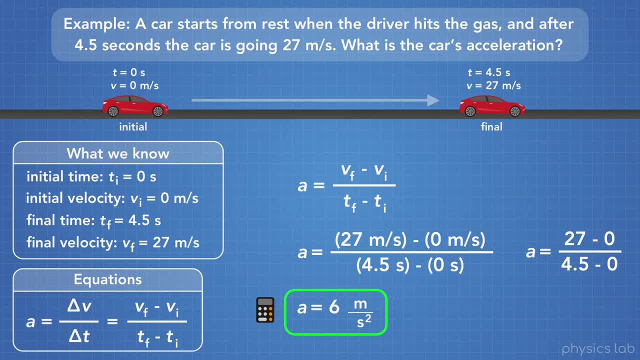 into this equation. So you might have asked: why did we have to use the right part of acceleration for acceleration? Could we have used the other part? acceleration equals change in velocity over change in time. Yeah, we definitely could have done that too. 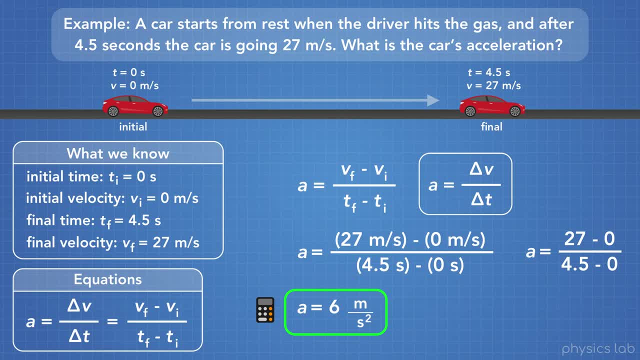 Instead of using initial and final values for velocity and time, we could have used change in velocity and change in time. We might have read the problem and thought: well, it starts at rest and speeds up to 27 meters per second, so the change in velocity. 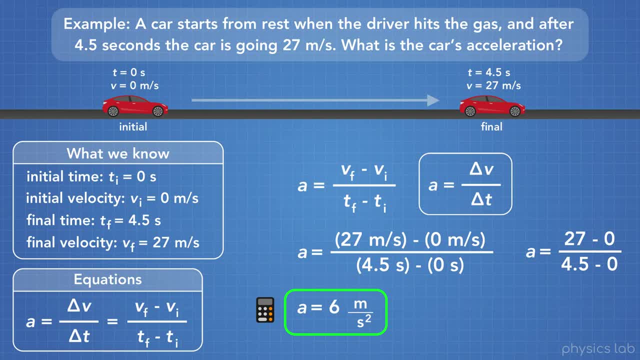 must be 27 meters per second, And it takes 4.5 seconds to speed up, so the change in time is 4.5 seconds. That way works too, And for this problem it seems simpler, But sometimes the car isn't starting at rest. 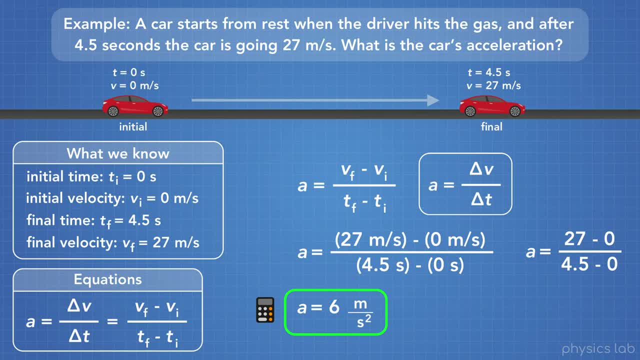 and the initial velocity isn't zero, And later on we'll learn that if the car is going the other way, the velocity is actually negative. So we would have to write out initial and final velocities anyway, just to keep track of everything. 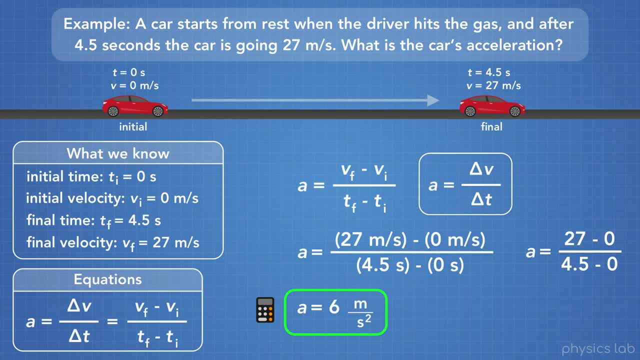 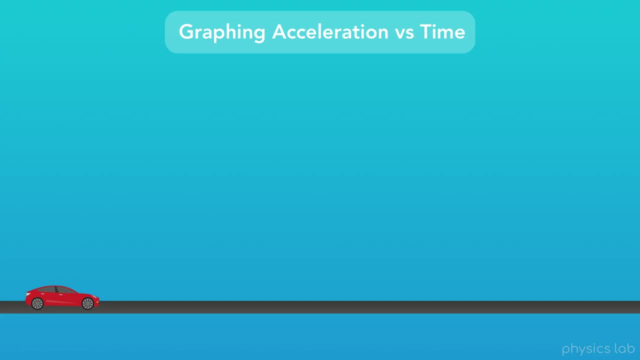 So long story short. initial and final values is a good habit to make sure we don't mess up, But for simple problems like this one, we don't need to Alright. so, just like we did with position and velocity, let's try to graph the acceleration. 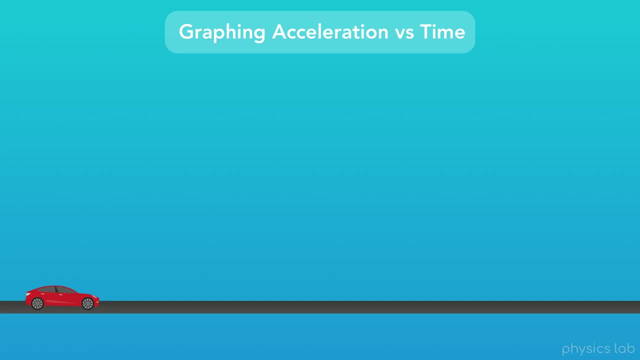 of a car over time. This is the new motion of the car. Like before, we can imagine a person in the car looking at the speedometer and writing down velocity of the car at different points in time, And this is what we get. 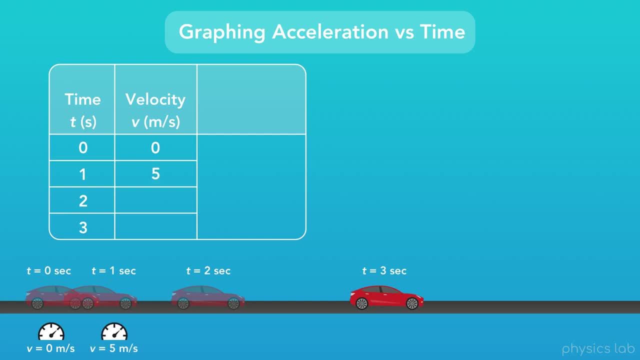 At 0 seconds, the velocity is zero and the car isn't moving. At 1 second, the velocity is 5 meters per second. At 2 seconds, the velocity is 10 meters per second, And at 3 seconds the velocity is 15 meters per second. 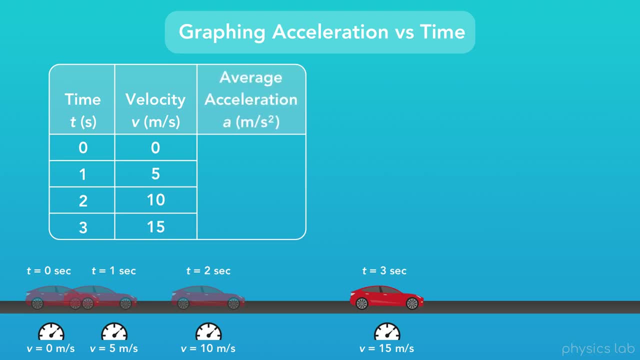 Now what we can do is calculate the average acceleration of a car between each pair of time points using our equation for acceleration, And I'll do the math for us. What we'll find is that the acceleration between seconds 0 and 1 is 5 meters per second squared. 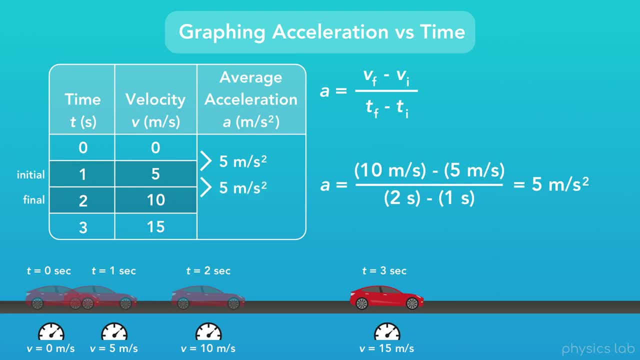 Between seconds 1 and 2, it's 5 meters per second squared, And between seconds 2 and 3, it's still 5 meters per second squared. So we can see that the velocity is increasing over time, but the acceleration of the car 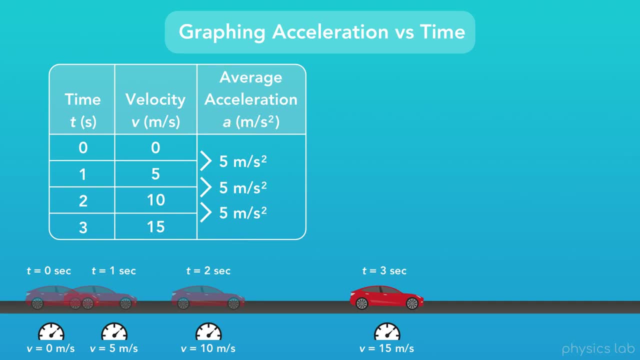 stays the same, And that makes sense. The car has some acceleration and acceleration is the change in velocity over time. So the car's velocity changes over time. So what would our graph of acceleration look like? As always, we have time along our horizontal axis. 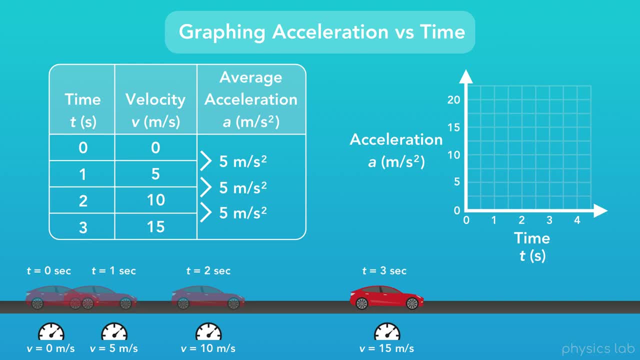 and now we have acceleration along the vertical axis For the period of 0 to 1 seconds. we know the acceleration is 5 meters per second. squared From 1 to 2 seconds, it's 5 again, And from 2 to 3 seconds. 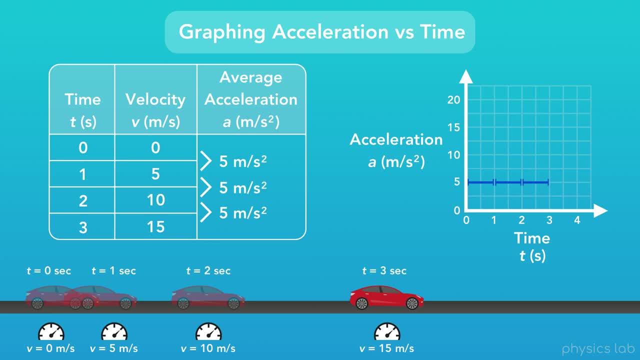 it's still 5.. And there we go. We have a graph of the car's acceleration over time. However, like we covered with velocity, this is just a graph of the car's average acceleration plotted across each time period. But could we do? 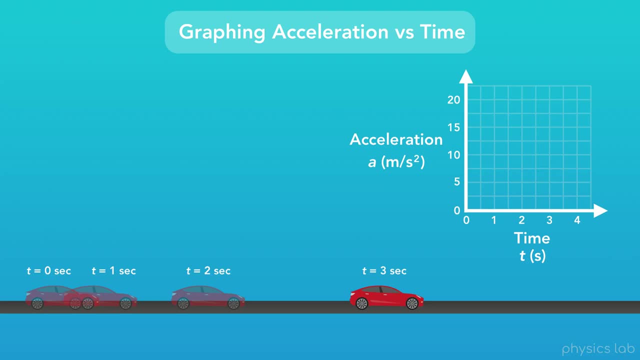 what we did with velocity. Instead of just calculating the average, could we measure the car's acceleration at different points in time? Actually we could. There are things called accelerometers which measure acceleration And, interestingly enough, you have one in your phone. 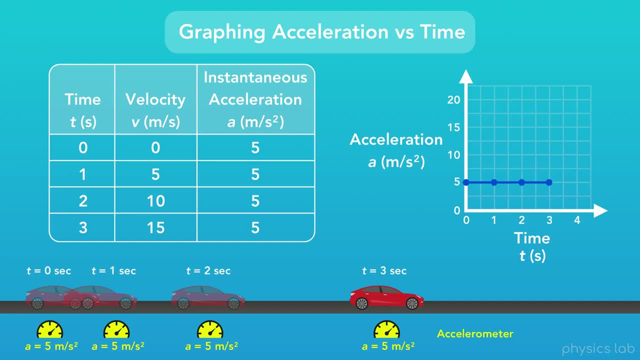 So, like we said, this car has an acceleration causing the car to speed up and the car's velocity to increase, but the actual value of acceleration doesn't change over time. In this course, and in most courses, this is as far as we're going to go. 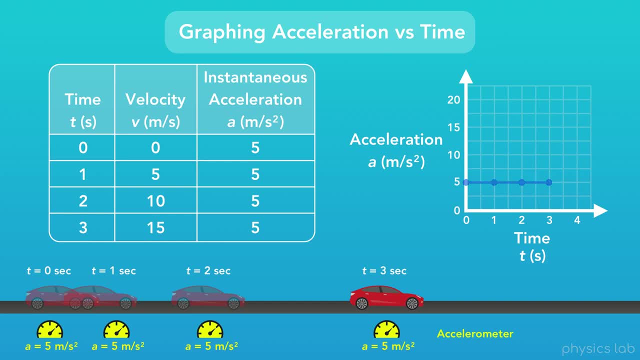 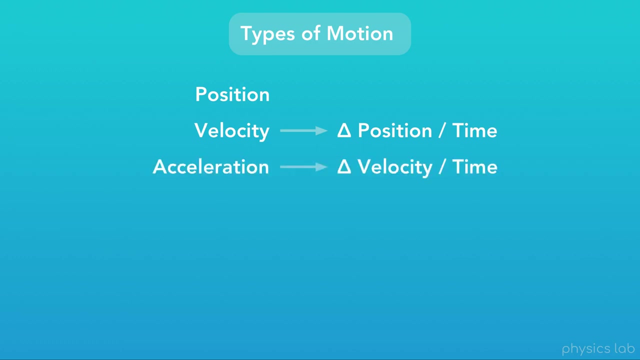 We won't deal with accelerations that change over time, But could we have an object with an acceleration that increases over time like this? Yeah, we actually could Just like: velocity is the change in position over time and acceleration is the change in velocity over time. 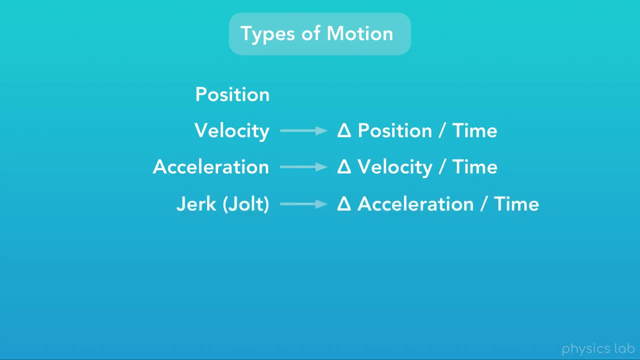 jerk or jolt is the change in acceleration over time, And it turns out that we could keep going. I just learned from googling this that the next steps would be a jounce or snap, a flounce or crackle. 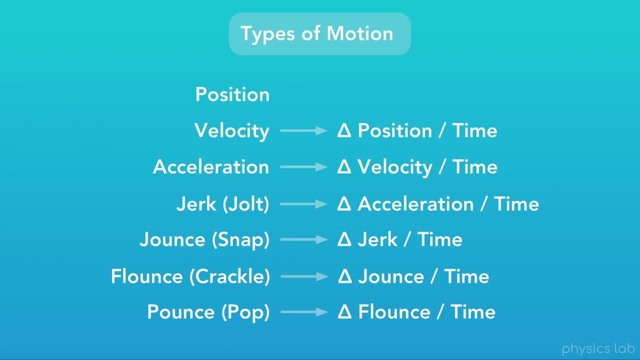 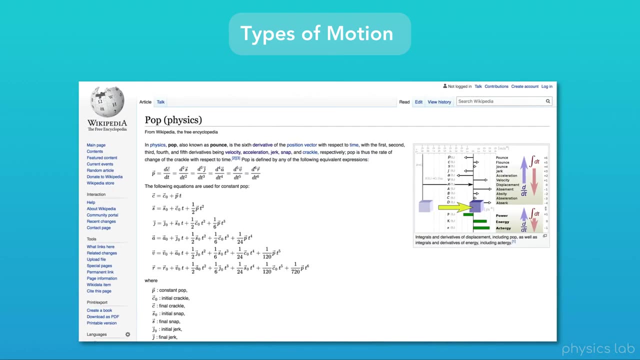 and a pounce or pop. This is not a joke. Jounce, flounce and pounce and snap, crackle and pop are all real physics terms. Look it up on Wikipedia. But yeah, for this course. 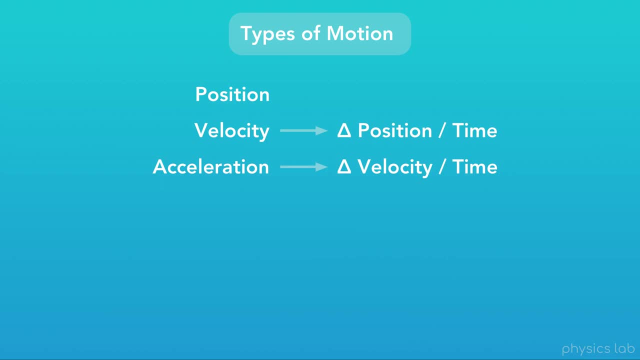 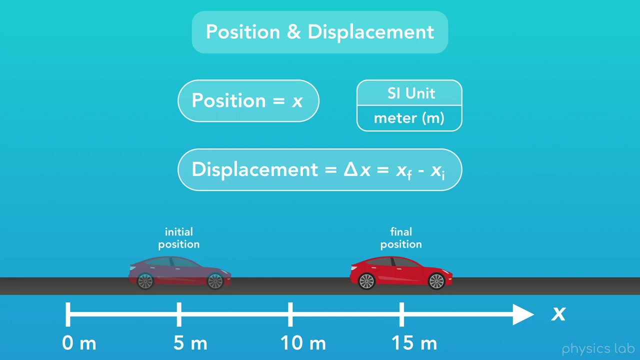 we're only going to work with position, velocity and acceleration. Alright, lots of stuff in this video. Let's do a recap. First, we learned about position, which has the SI unit of meters, and displacement, which is the change in position. 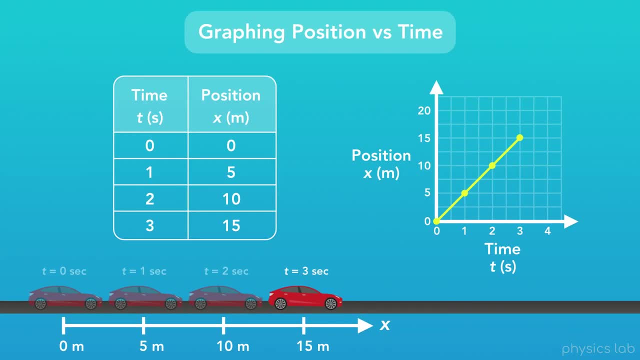 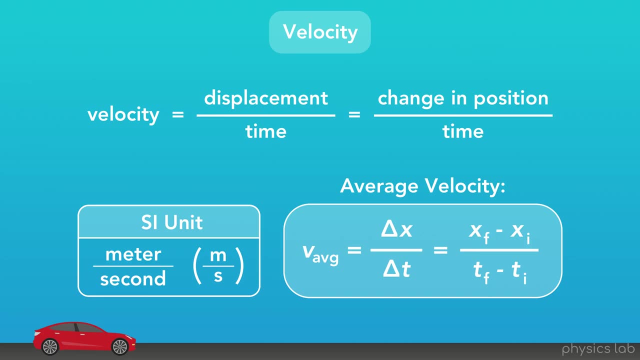 We also learned how we can graph an object's position over time. Next, we learned about velocity, which is the displacement over time or the change in position over time. The SI unit for velocity is meters per second, and we learned the equation for average velocity. 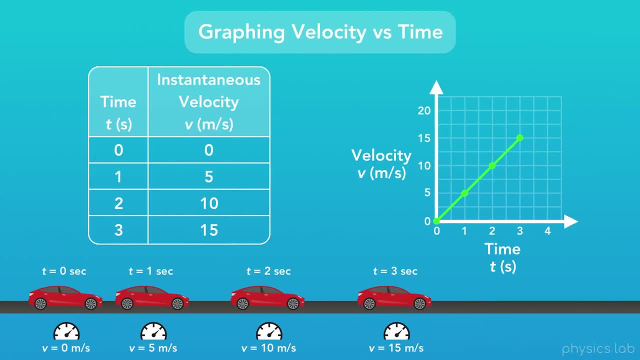 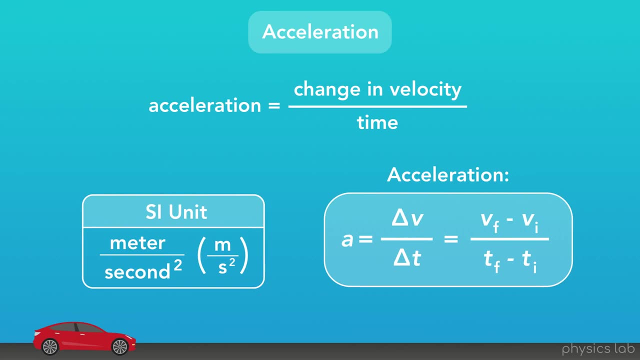 We also learned that we can measure and graph an object's velocity over time. And last, we learned about acceleration, which is the change in velocity over time. The SI unit for acceleration is meters per second squared, and we learned the equation for calculating acceleration. 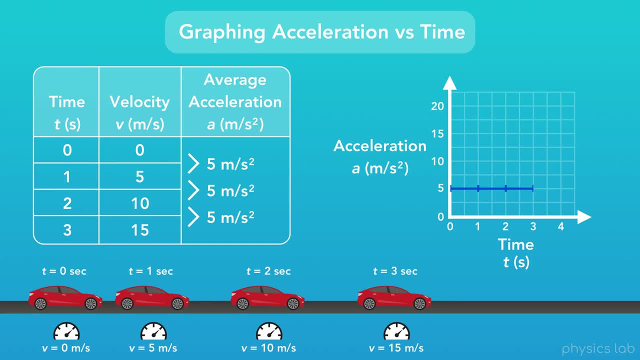 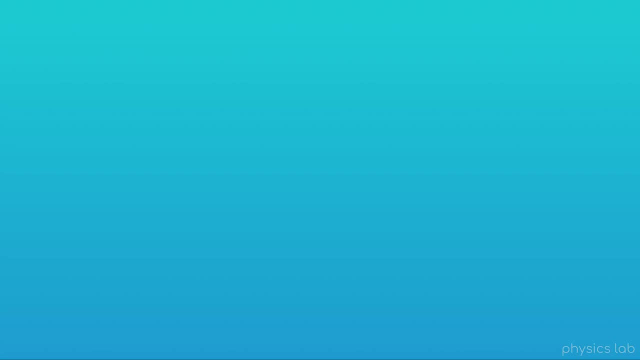 And finally, we learned how we can graph the acceleration of an object over time. So thanks for watching. I'll see you in the next video and we'll learn more about linear motion.